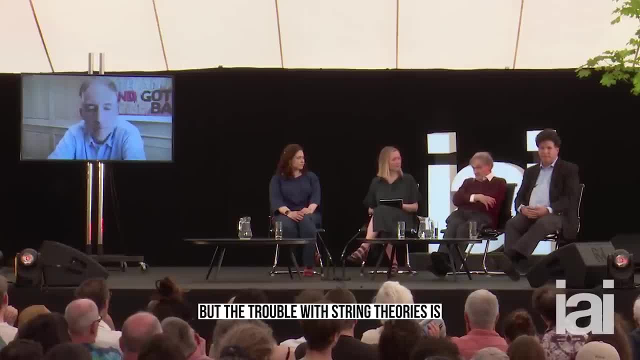 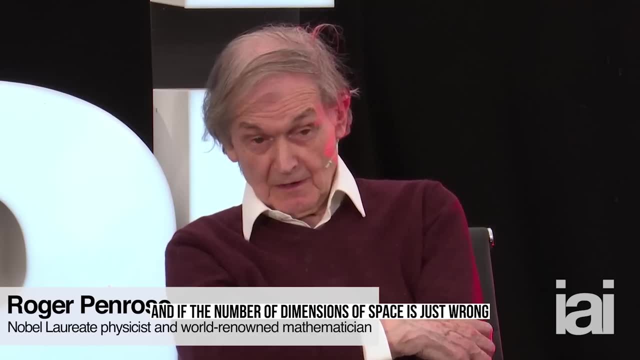 A lot of what I do is driven by the mathematics. But the trouble with string theory is it's supposed to be a theory of the way the world operates, And if the number of dimensions of space is just wrong, I can't take it seriously. 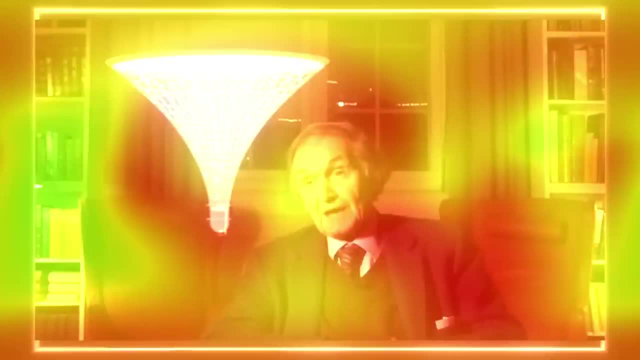 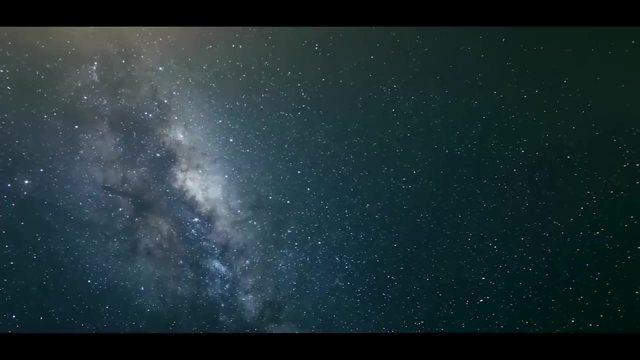 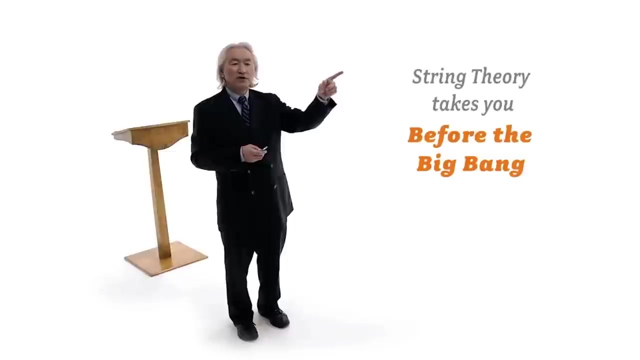 British mathematician and philosopher, Sir Roger Penrose, and American theoretical physicist Michio Kaku are two prominent figures in the scientific community. Sir Roger Penrose is famous for his research on black holes and Michio Kaku is renowned for his string theory. 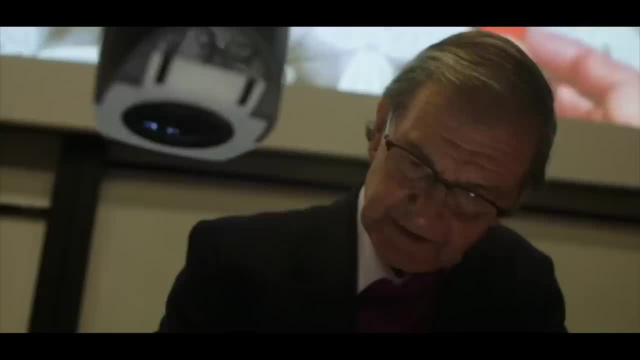 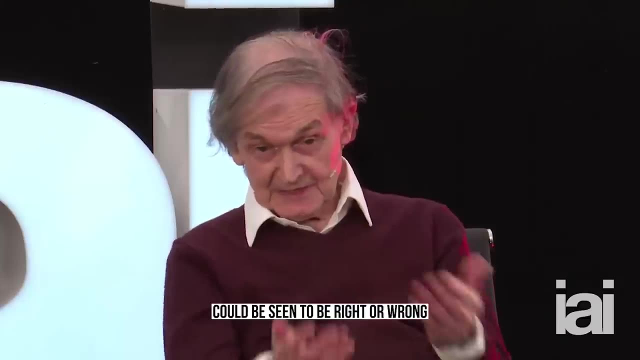 However, did you know that Sir Roger Penrose strongly rejects Michio Kaku's string theory? If you could have a theory which had predictions and these predictions could be seen to be true, and these predictions could be right or wrong. that's what I understand about physics. 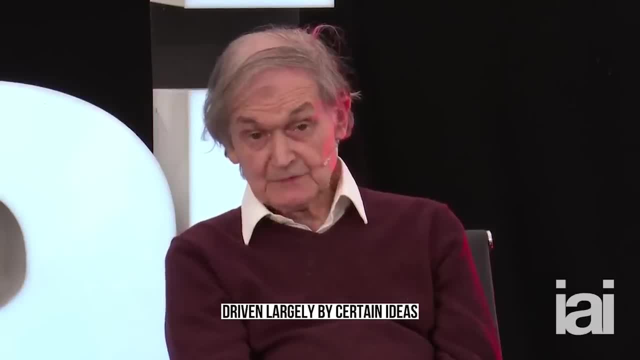 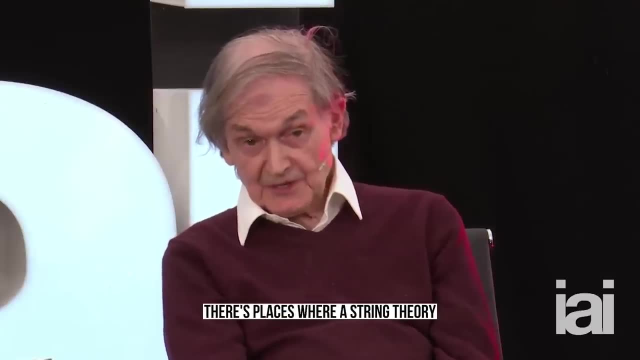 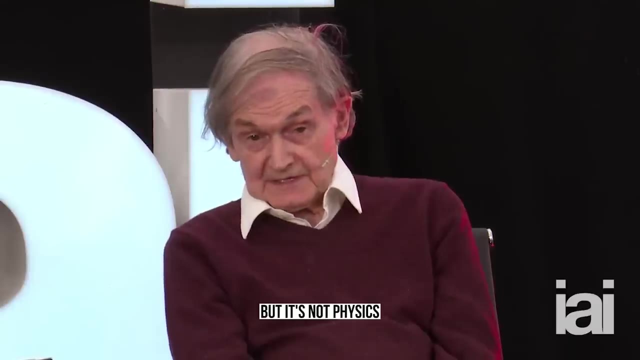 But string theory seems to me driven largely by certain ideas which have importance in mathematics but are sort of irrelevant to the physics. really, As far as I know, there are places where string theory has had an impact on mathematics. Sure it has, but it's not physics as far as I can see. 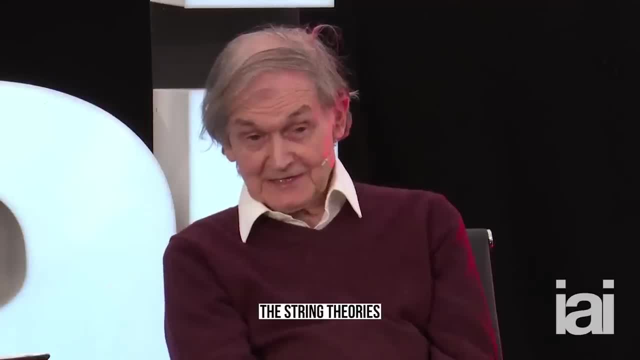 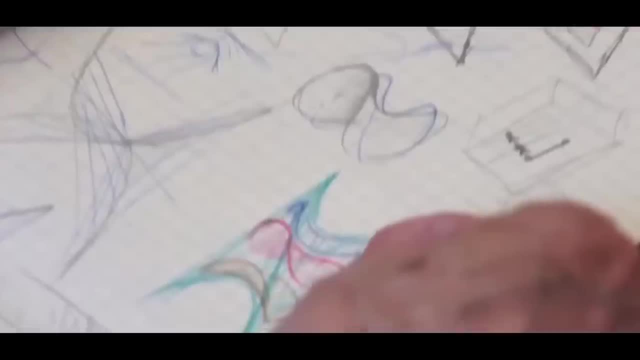 So the main trouble I have with string theory is: I don't think it's physics. What's more interesting is that Sir Roger Penrose. Sir Roger Penrose- doesn't even believe in the idea of cosmic inflation and suggests that cosmic inflation is nothing more than a fantasy. 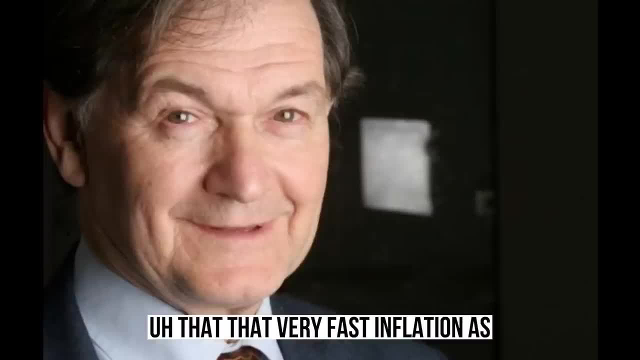 For example, you refer to inflation, very fast. inflation as a fantasy. Do you still believe that? Well, I've been trying to write a book for about ten years for the Princeton University Press, called Fashion, Faith and Fantasy in the New Physics of the Universe. 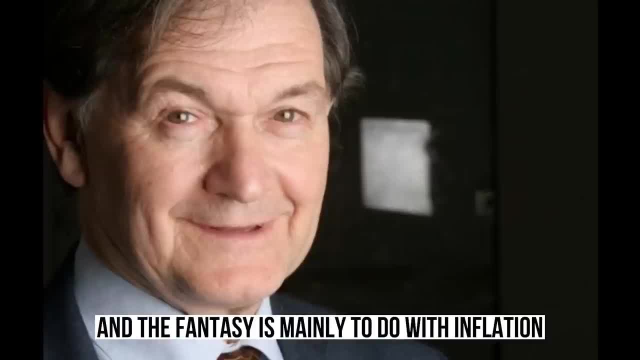 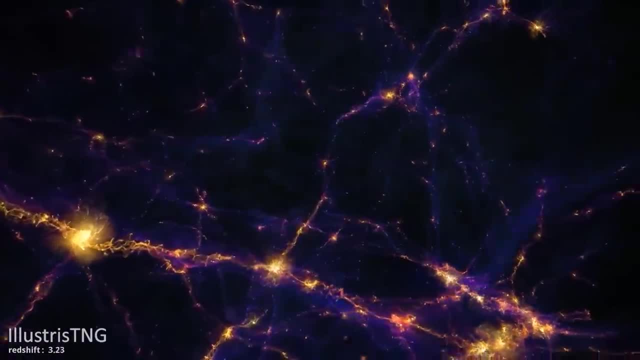 And the fantasy is mainly- It's mainly to do with inflation. that's true. Dark matter is important for explaining certain phenomena in the universe, but scientists believe that dark matter might not even exist. So why does Roger Penrose reject Michio Kaku's string theory? 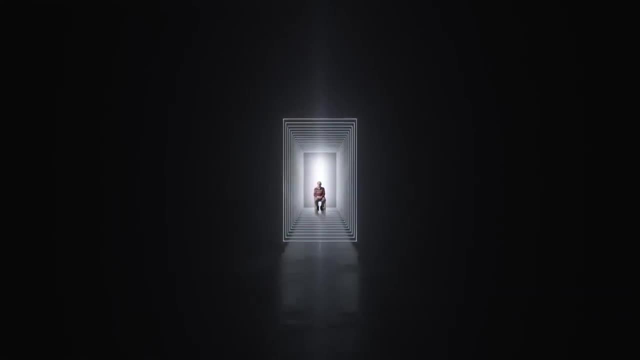 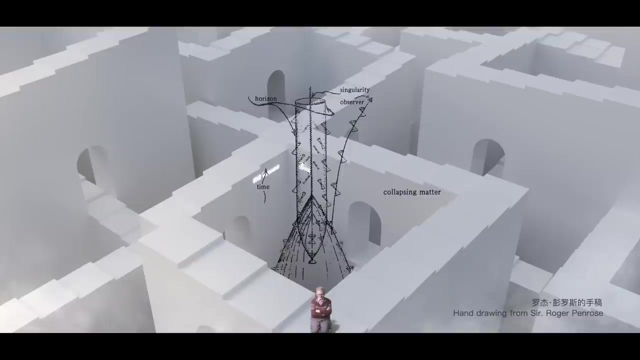 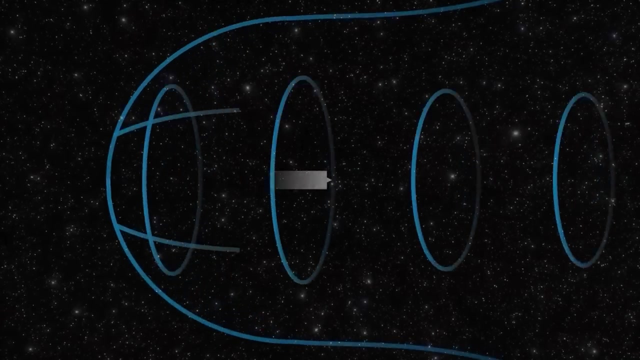 Why does he say that cosmic inflation is a fantasy? What groundbreaking research has Sir Roger Penrose conducted on black holes, and why are scientists still uncertain about the existence of dark matter? Let's dive in to find out. Our universe is composed of matter which, upon closer examination, consists of particles. 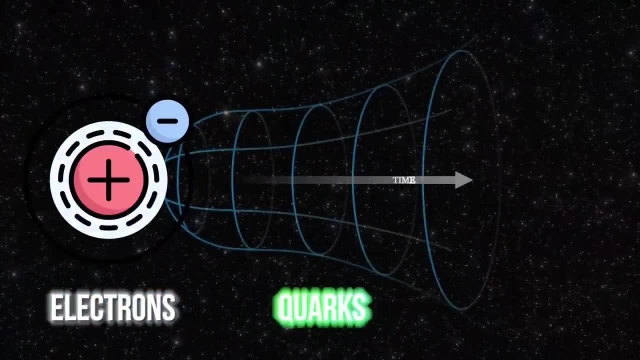 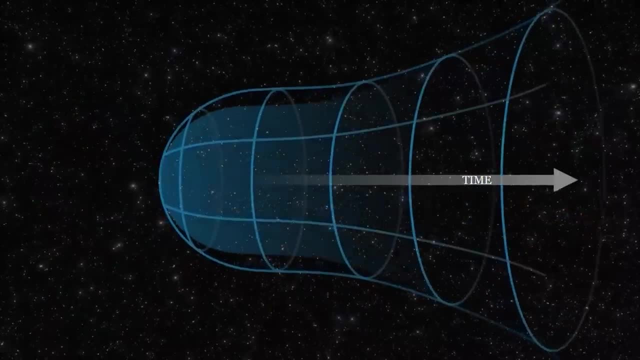 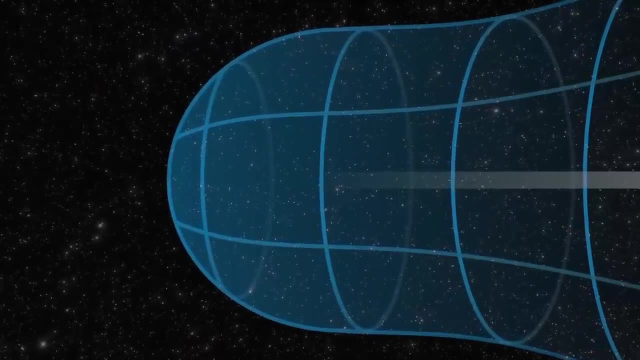 These particles come in various types, such as electrons, quarks and neutrinos. They move throughout the universe and can interact by exchanging other particles. For instance, the exchange of photons mediates the electromagnetic force. All these distinct particles are accounted for in what we refer to as the Standard Model. 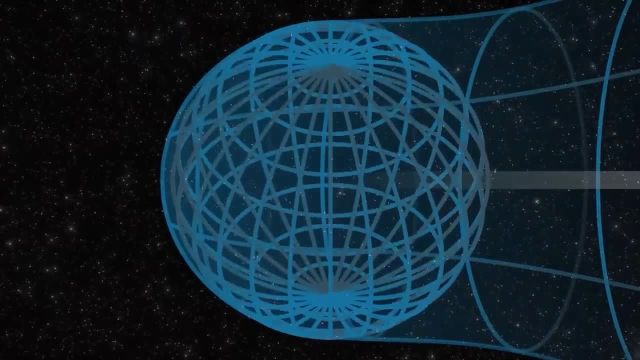 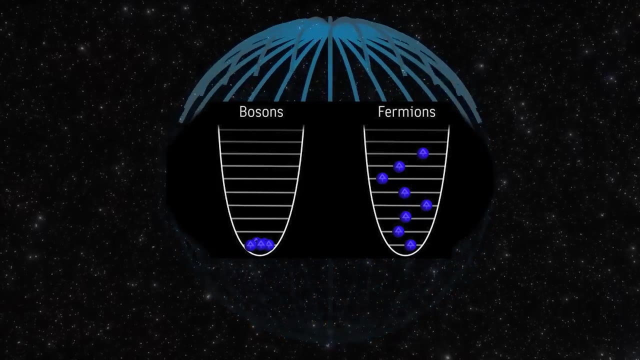 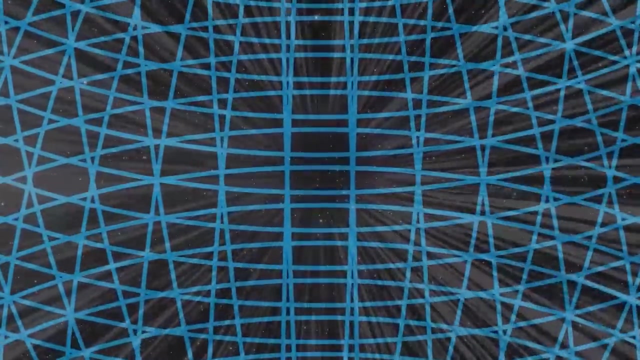 which is presently our most precise mathematical description. It encompasses two primary categories of particles: fermions, which primarily constitute matter, and bosons, which mainly describe interactions. At first glance, one might assume that this is the ultimate theory, that the Standard Model encompasses everything. 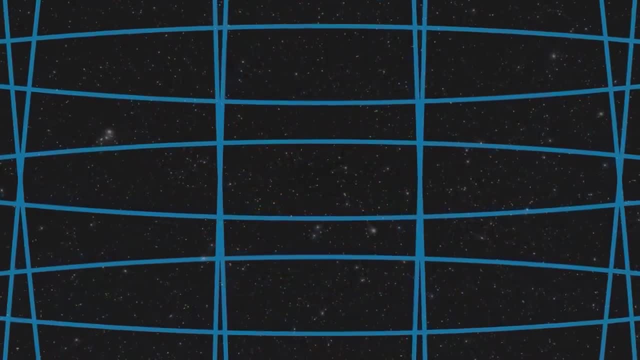 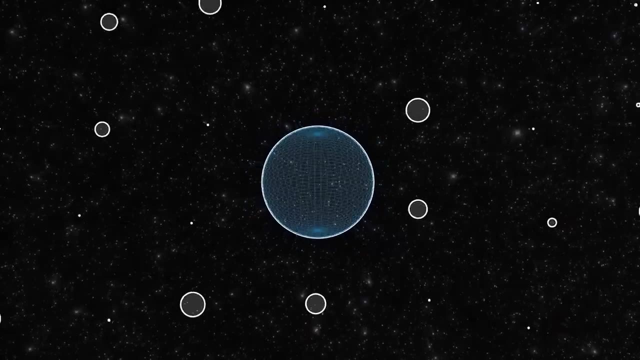 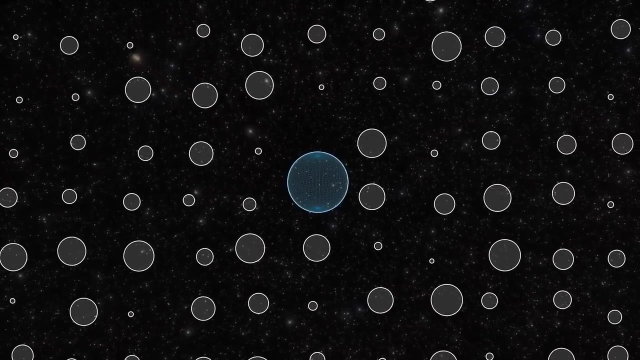 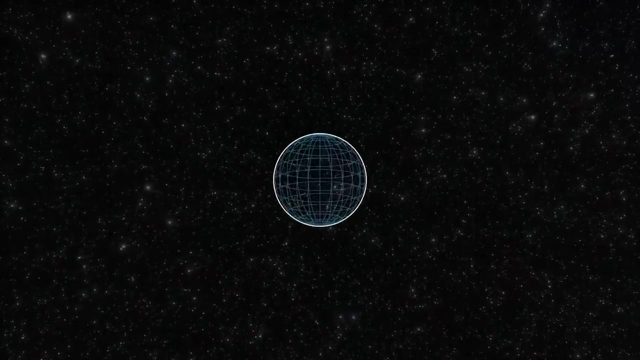 However, there is an interaction that this model unfortunately fails to account for: gravity on a large scale. We know that general relativity describes gravity. objects curve space-time, thereby attracting other objects. Similar to other types of interactions, we anticipate that the curvature of space-time consists of small particles at the quantum scale called gravitons. 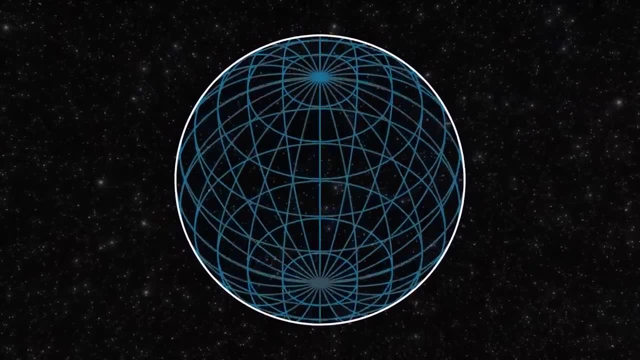 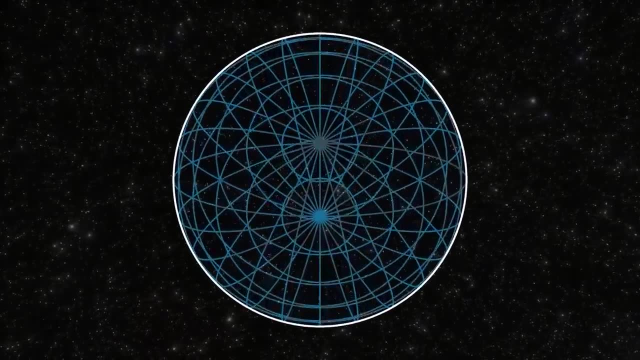 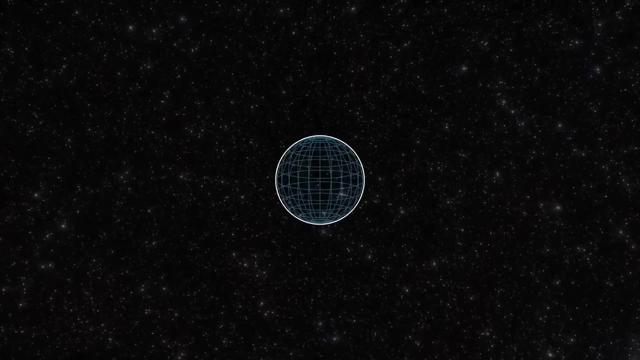 which are quanta of space-time curvature. Nevertheless, when we attempt to incorporate their graviton into the Standard Model, the calculations yield absurd results with infinite values that cannot be eliminated. We are unable to describe gravity at the quantum scale. To tackle this predicament, 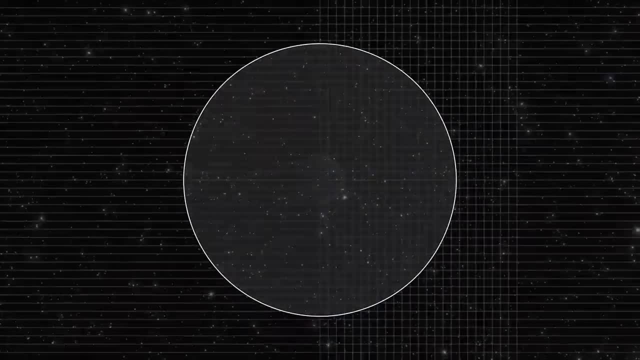 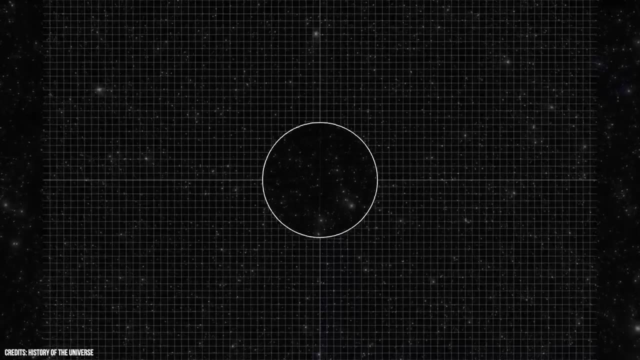 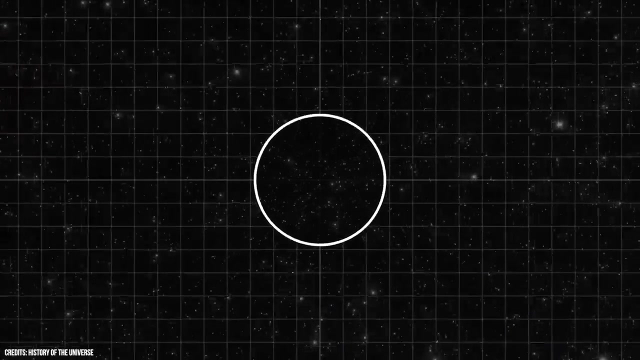 physicists have been searching for new theories for over half a century. This is where the String Theory comes in. The basic concept of the String Theory is quite simple. In the Standard Model, particles are depicted as dimensionless points. We acknowledge that these points do not possess identical properties. 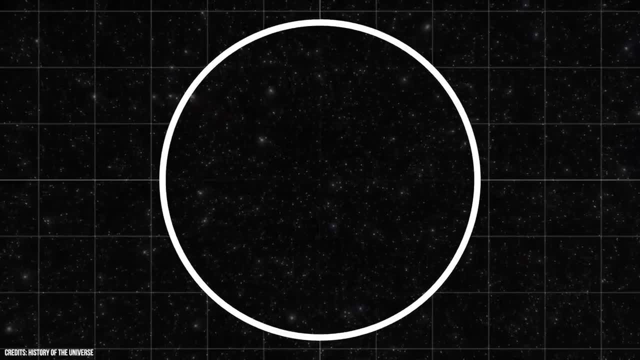 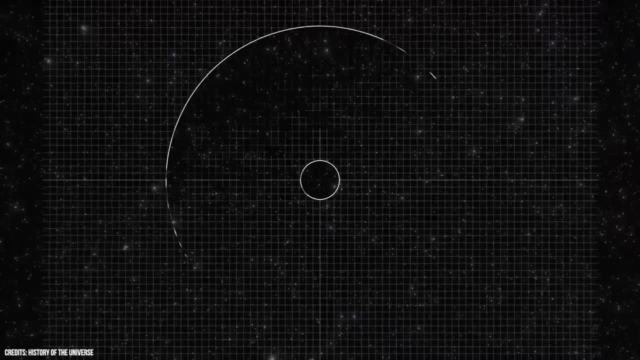 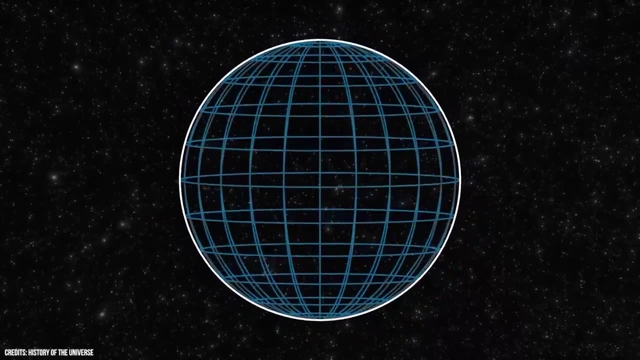 In String Theory we assume that this is merely an approximation. If we zoom in on the particles, we postulate that they are all composed of tiny strings, sometimes open and sometimes closed. These minuscule strings possess tension akin to tiny rubber bands. 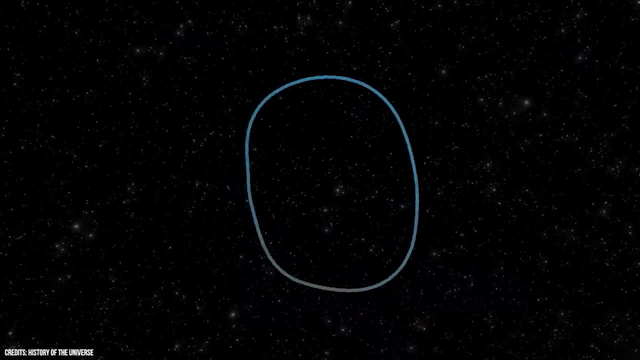 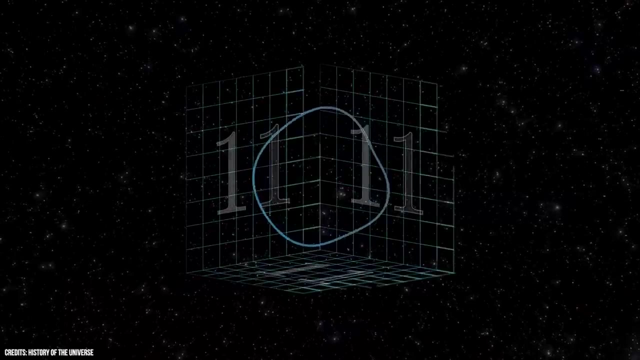 and they are capable of vibrating. A guitar string can vibrate in different modes or harmonics. Likewise, our little strings can vibrate in various ways: one ripple, two ripples, three ripples and so forth. The different vibrating modes behave on our scale. 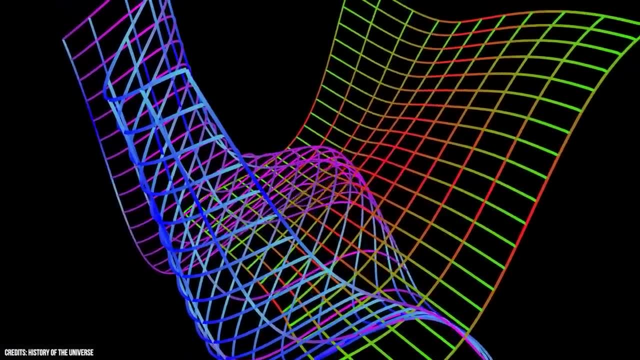 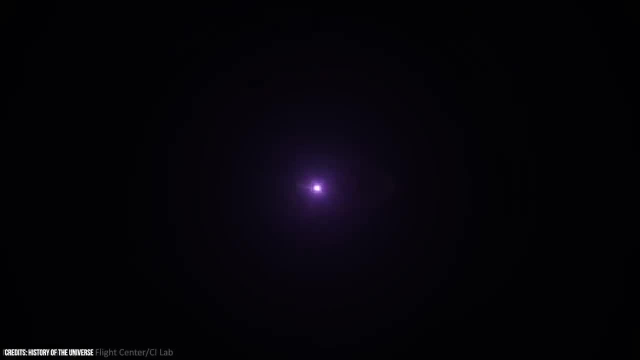 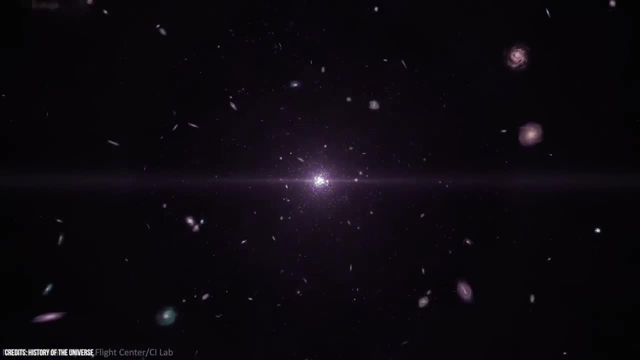 as distinct types of particles. Through these calculations, we discover that certain strings behave like photons and, even more remarkably, some behave like gravitons. By starting from the fundamental premise that particles are tiny strings with tension, we already explain the existence of different particle types. 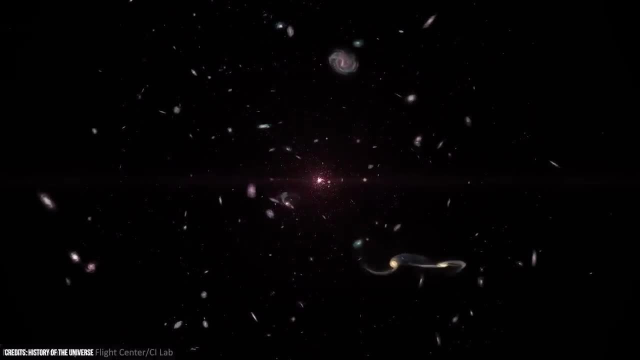 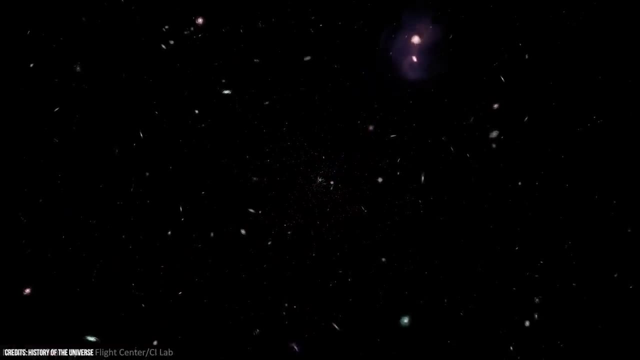 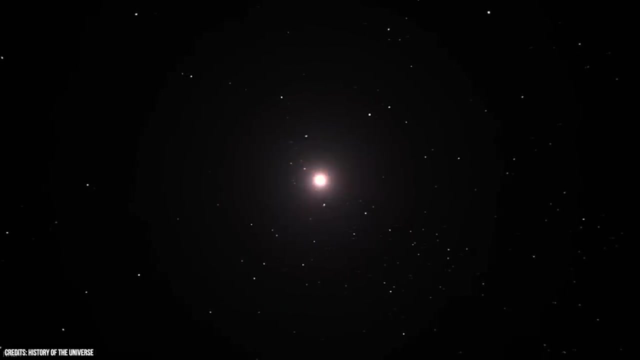 and naturally predict the presence of the graviton, thereby describing gravity at the quantum scale. Now let's delve into understanding how these strings evolved within the Universe. To accomplish this, we'll employ the same principles as our current models. Imagine we launch an electron towards a target. 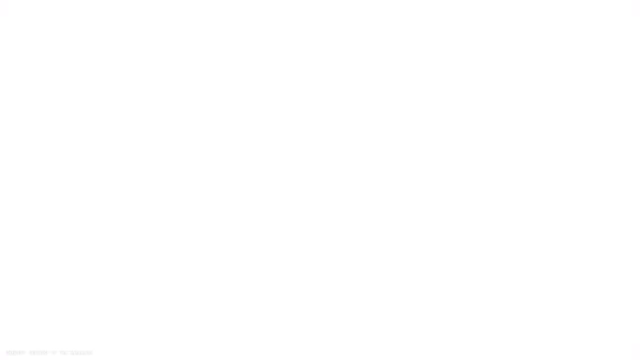 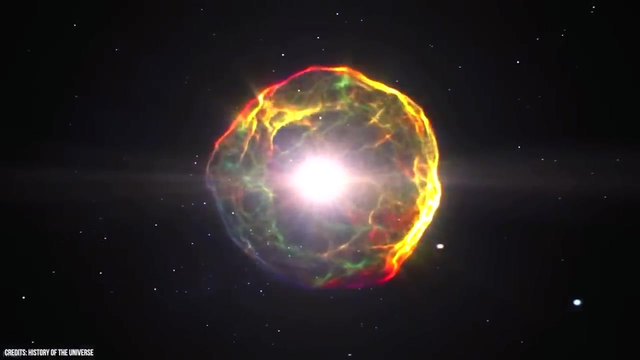 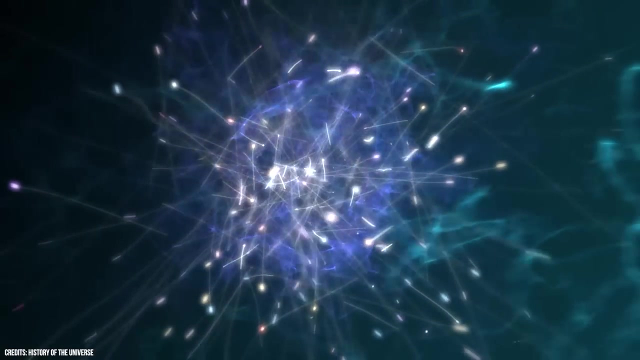 The electron propagates like a wave, and when it reaches the target, we cannot precisely determine where it will manifest. At the quantum scale, the same experiment can yield different results. We can only predict the probability of observing specific outcomes, and the aim of physics at this scale is to ascertain these probabilities. 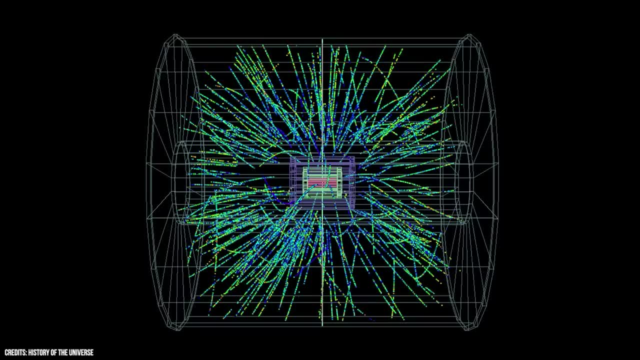 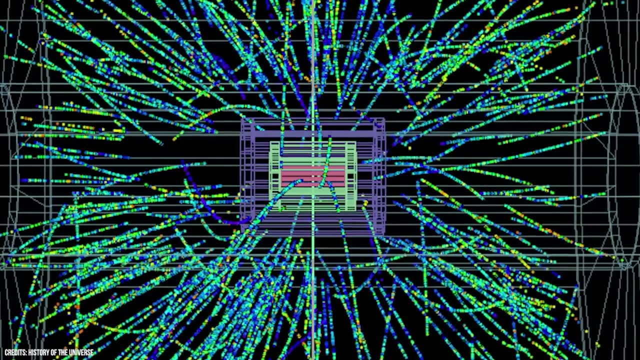 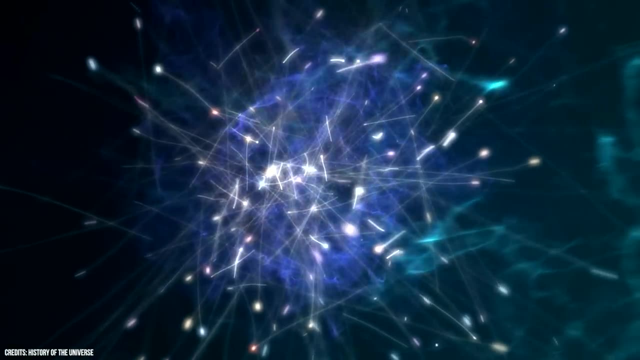 The mathematical approach for determining the probability of observing a particular result involves considering all possible scenarios that lead to it. Simultaneously, we sum up all trajectories and all potential interactions. For instance, an electron can emit a photon, then reabsorb it. 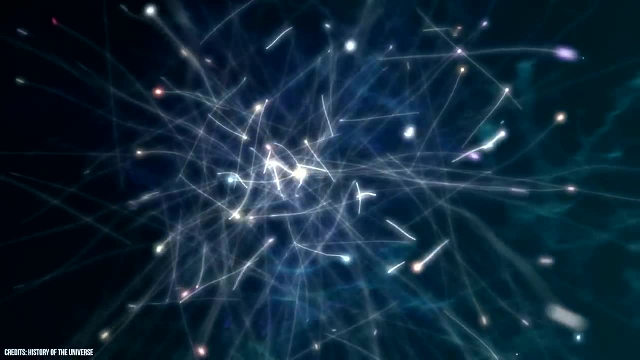 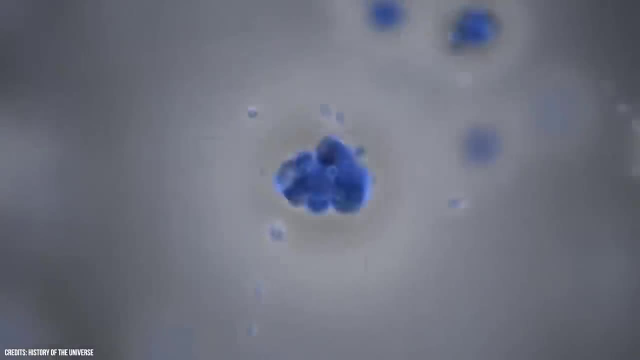 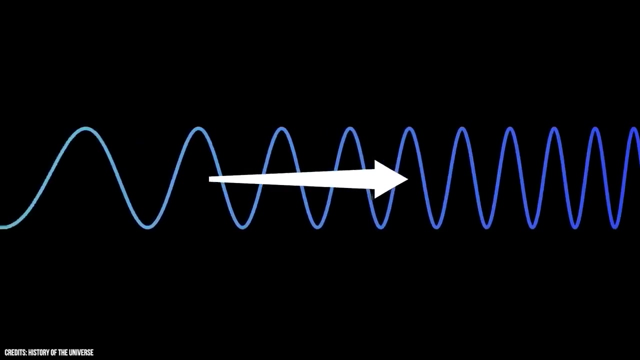 or emit two or even three photons. Within the scenarios we consider, we manually decide to allow specific types of interactions to reproduce what we observe in reality. By summing up all these scenarios, we obtain the desired probability. In string theory, the approach remains the same. 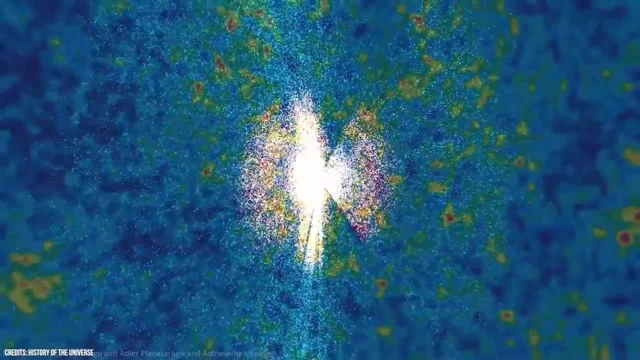 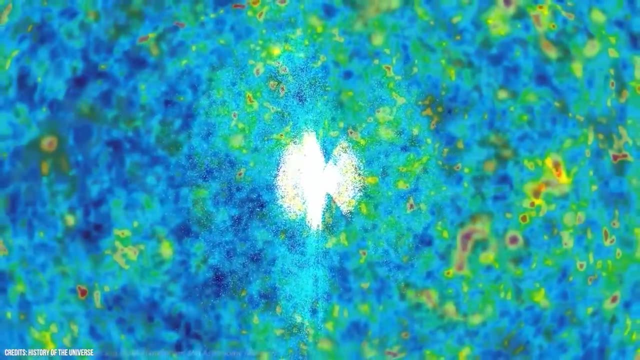 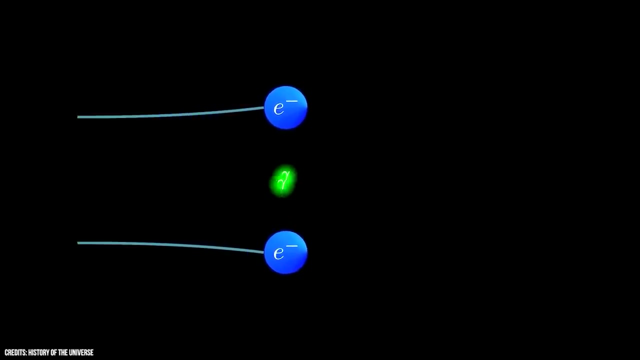 However, particles are no longer depicted as points. Whereas a point traces a trajectory over time, a string traces a surface. To describe the probabilistic evolution of a string, similar to quantum physics, we consider all possible geometries that the string can trace over time. 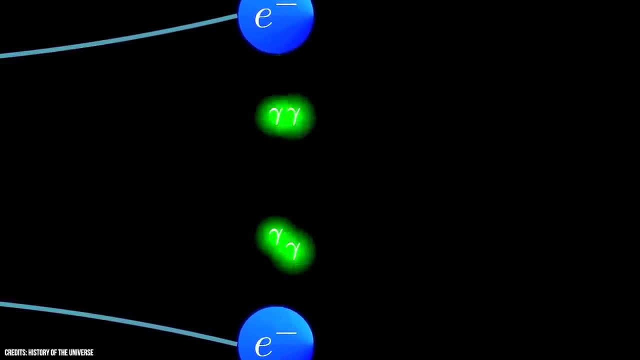 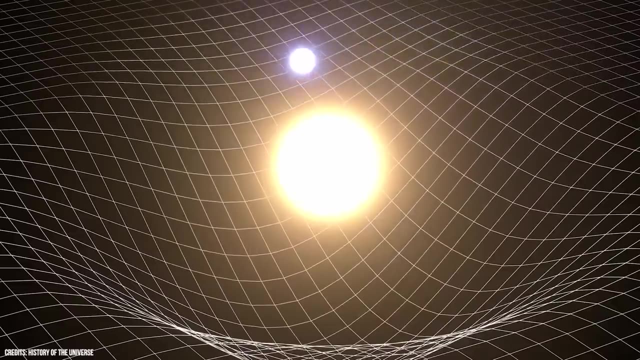 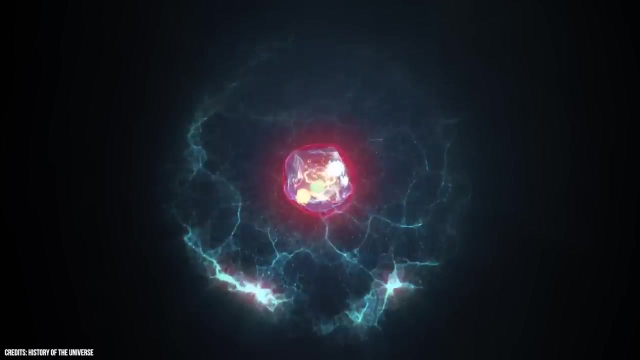 It may follow a specific trajectory, vibrate in a certain manner, duplicate itself or recombine, thereby forming a geometry with a whole. By summing up all possible geometries, string theory inherently incorporates interactions without requiring manual addition As a side note. 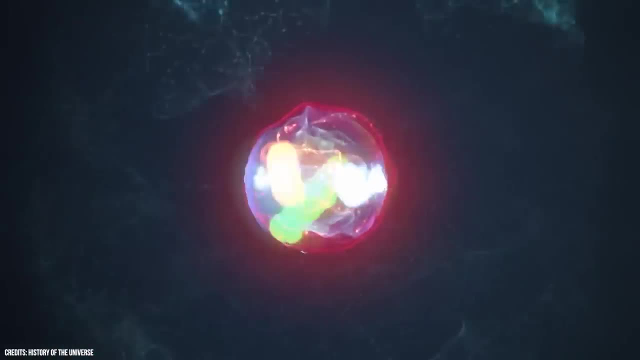 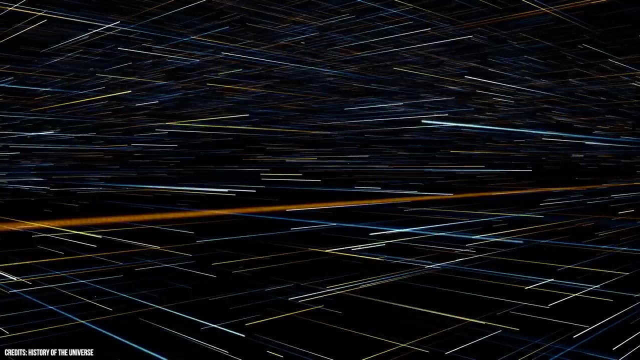 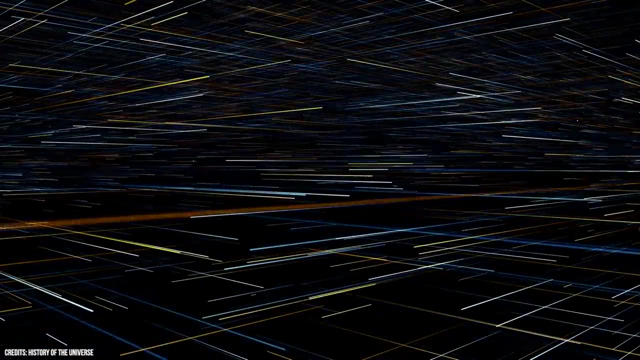 interactions in the standard model were considered to be local. For instance, the emission of a photon was instantaneous. In string theory, interactions are continuous. Particles are no longer instantaneously emitted but rather gradually. This resolves the infinities we encountered. 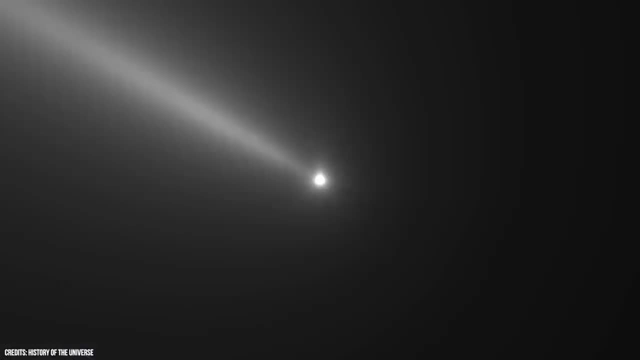 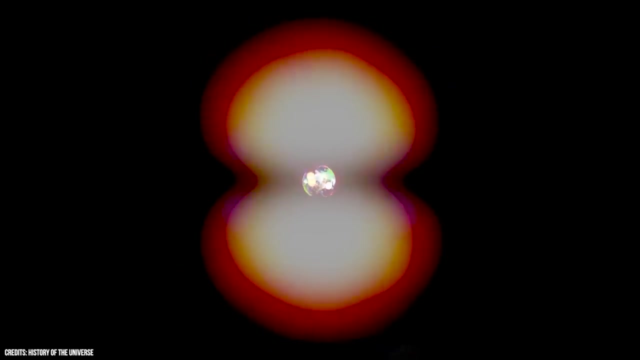 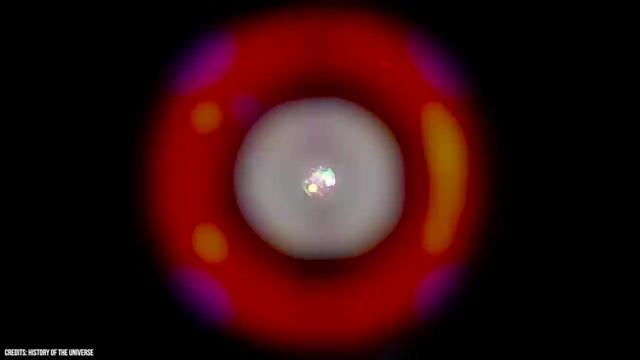 when attempting to include the graviton in the standard model. Consequently, string theory not only predicts the existence of the graviton, but also enables us to calculate its interactions with other particles and consequently describe quantum gravity. The theory so far appears very promising. 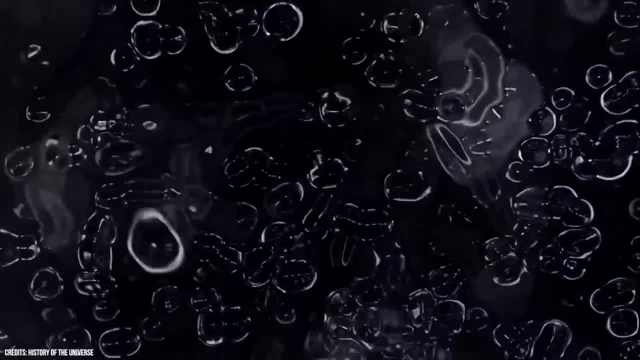 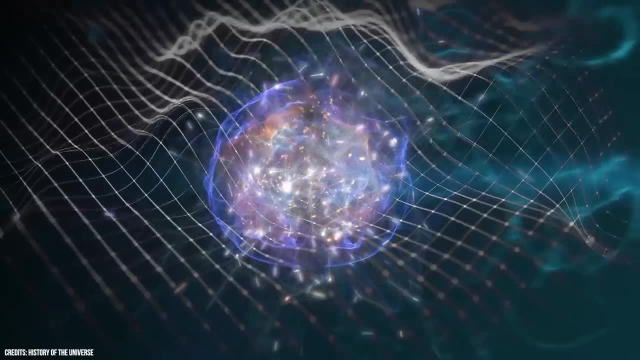 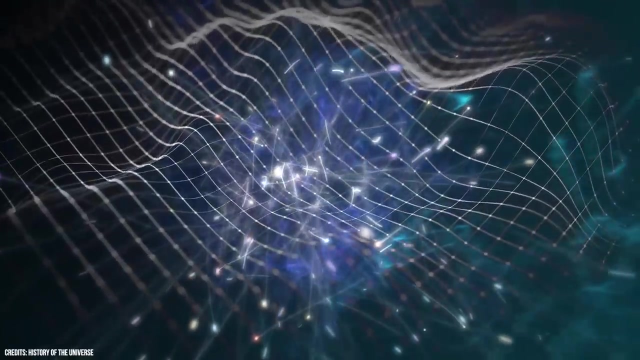 explaining the existence and interactions of different particle types. It even incorporates a quantum description of gravity. Unfortunately, at this stage, the model encounters three problems. The first problem is that all strings behave as bosons, like photons or gravitons. However, 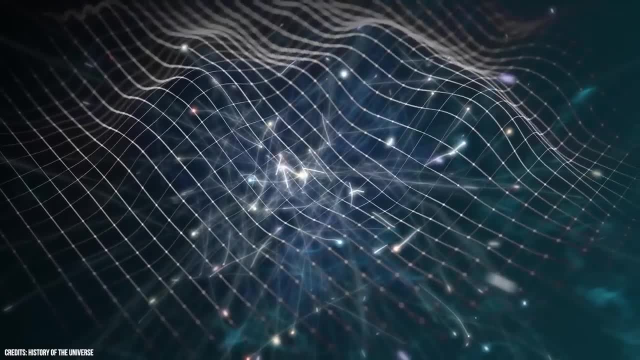 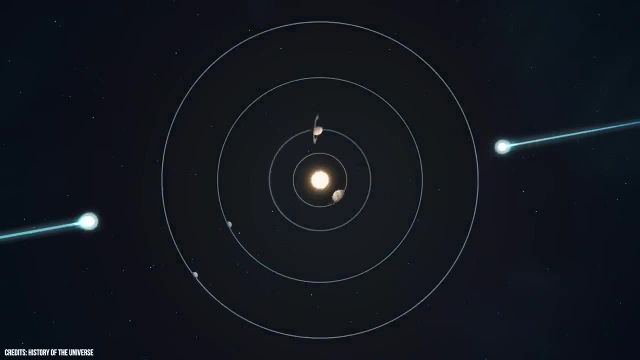 fermions like electrons, which exist in our world, are not predicted by our model. The second problem is the existence of a particle called a tachyon, which has a mass that seems to be an imaginary number, a mathematical issue that needs resolution. 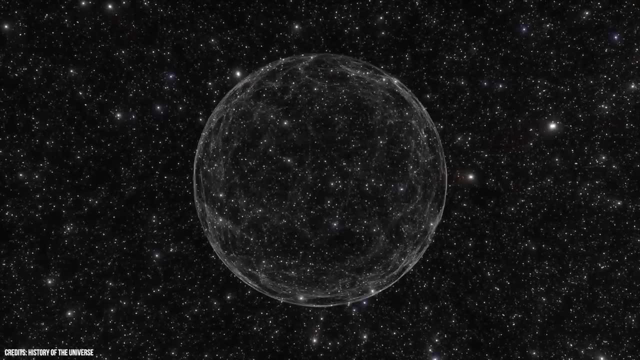 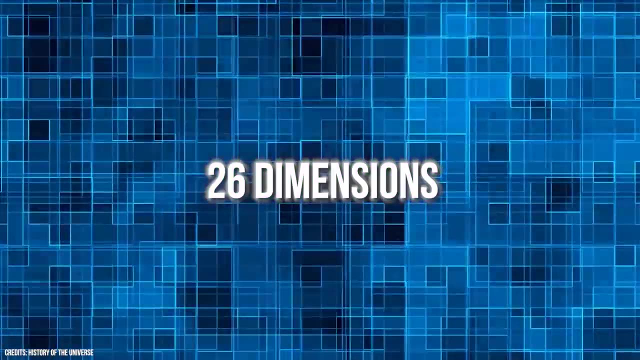 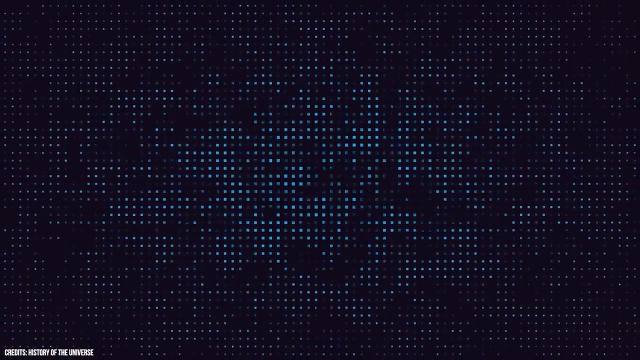 Lastly, our space-time comprises of four dimensions, three spatial and one temporal. However, this theory seems to only function in a universe with 26 dimensions. At present. string theory seems far from describing our universe. To address these issues, we need to push the theory further by incorporating fermions. 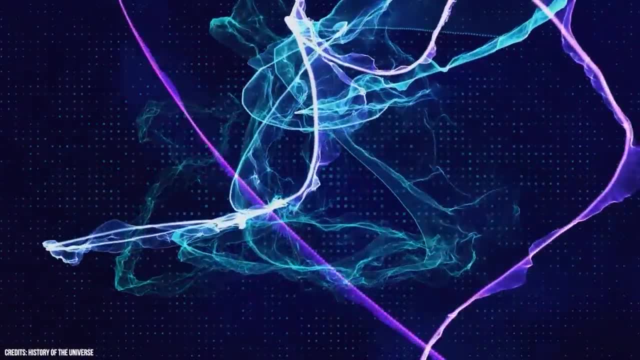 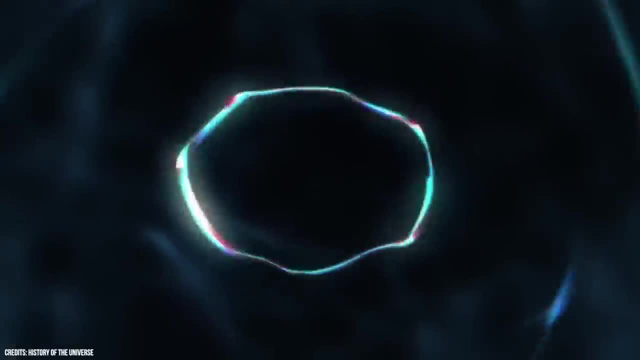 The idea is to introduce spinners on the strings which mathematically describe fermions in the standard model. By including spinners, we solve two problems: The model predicts the existence of fermions and it no longer predicts the problematic tachyon. 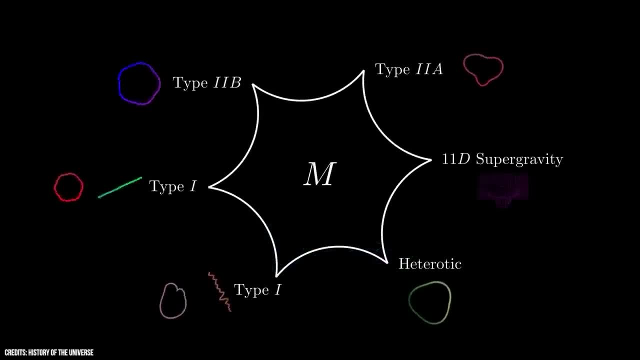 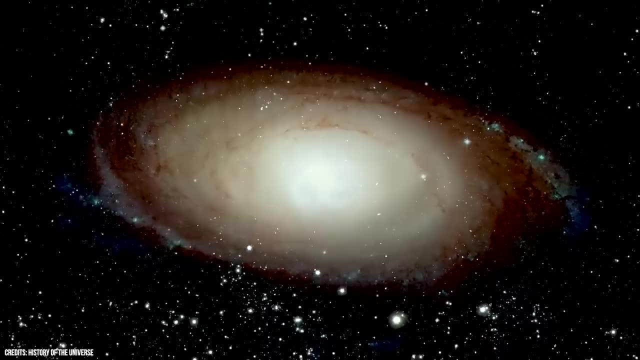 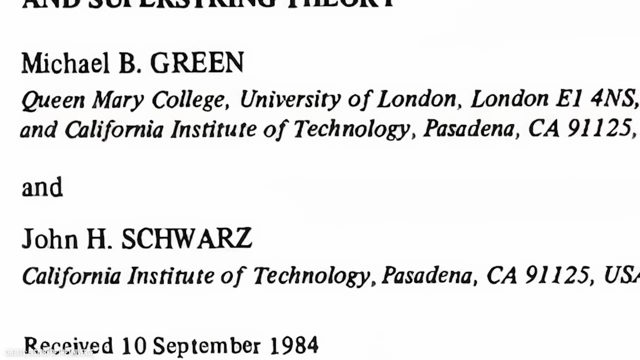 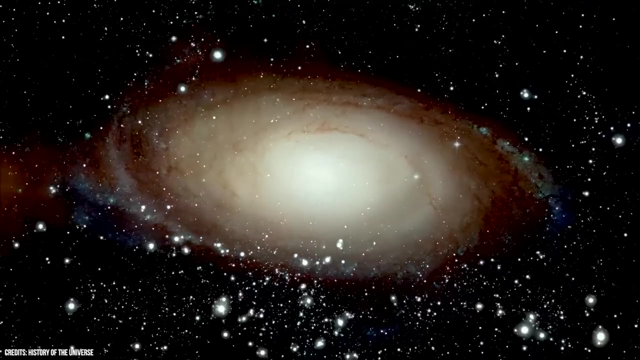 This more comprehensive theory is known as superstring theory. With the addition of spinners, it exhibits a fundamental symmetry between fermions and bosons, implying an equal number of each. This symmetry is called supersymmetry. But what about the third problem? 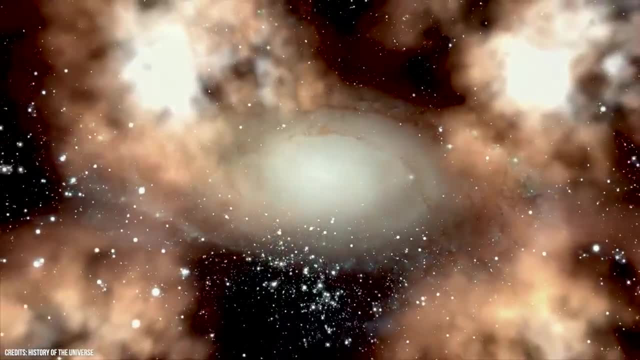 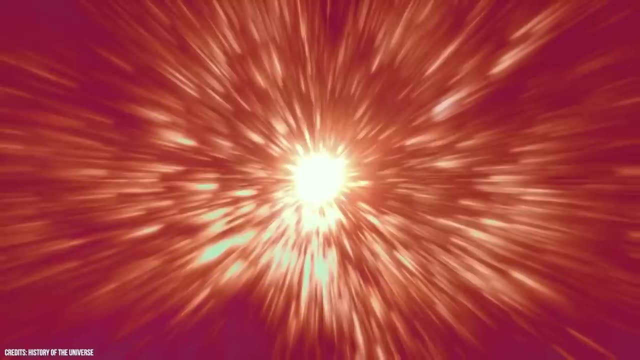 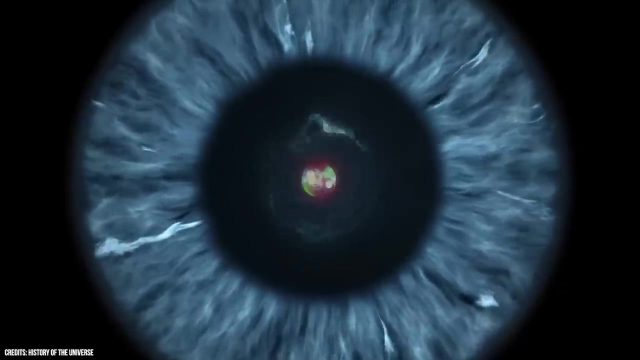 Before supersymmetry, the math required a 26-dimensional universe. Now superstring theory suggests a universe with 10 dimensions. Unfortunately, this third problem remains unresolved: The theory doesn't align with our 4-dimensional universe. Nevertheless, despite its shortcomings, 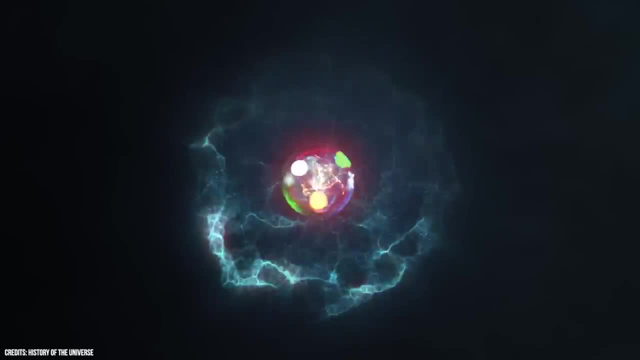 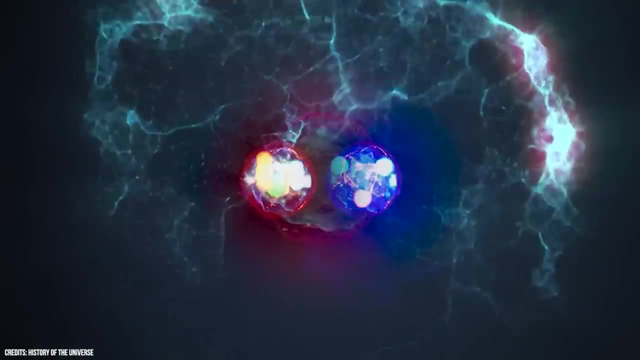 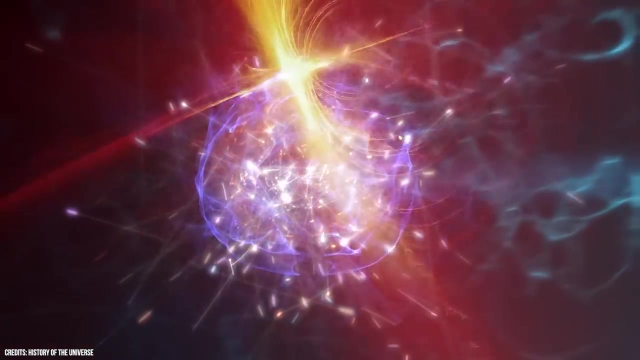 the model has shown great promise. Should we abandon it entirely? If the six missing dimensions exist, where might they be? One possibility is that our universe is a 3-dimensional slice of a larger 9-dimensional universe. Alternatively, the six unobserved dimensions. 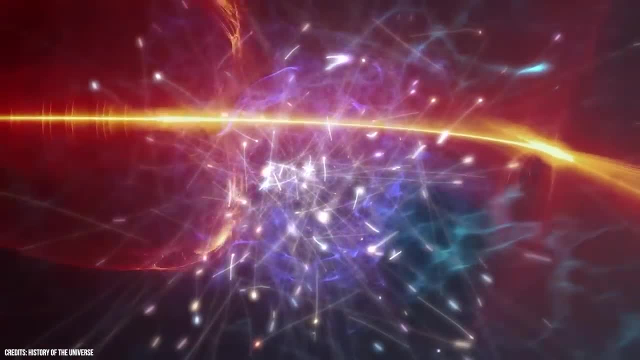 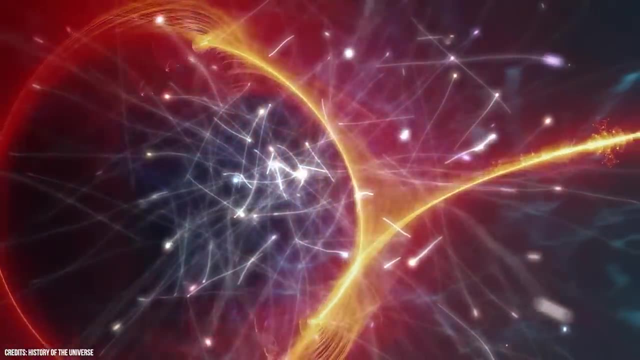 could be curled up on themselves. To illustrate, consider an ant walking on a straw. The straw has two dimensions and the ant can move back and forth and left to right around its circumference Zoomed out. we only perceive one dimension, while the second dimension 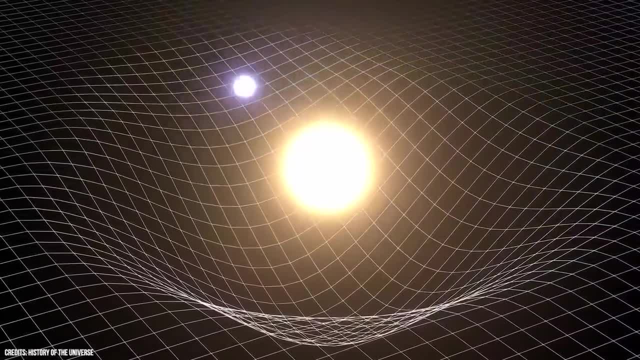 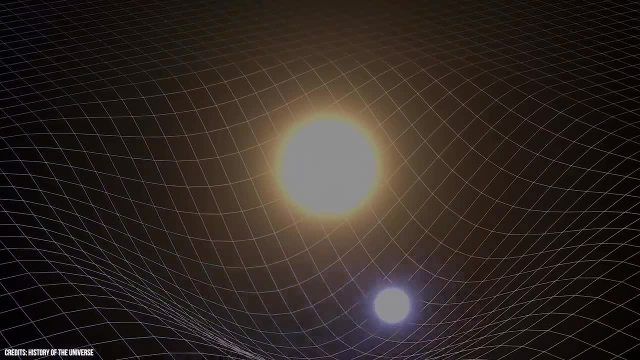 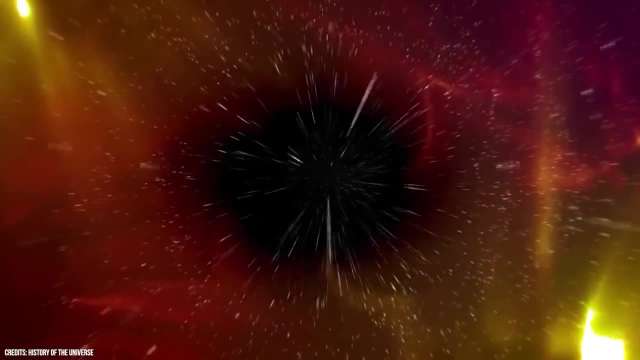 curled around the straw, remains minuscule and imperceptible. String theory suggests a similar phenomenon. Our universe would possess 9 spatial dimensions, but 6 would be compact and too tiny to observe at our scale. This hypothesis may seem far-fetched. 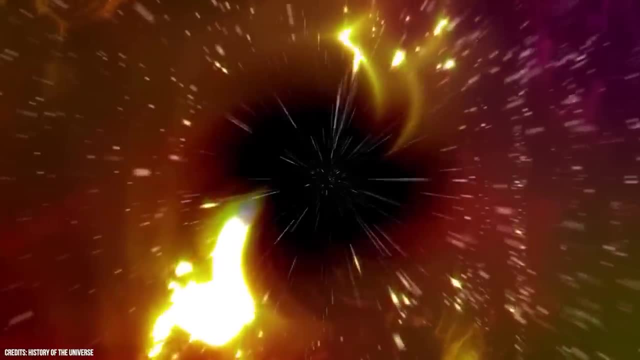 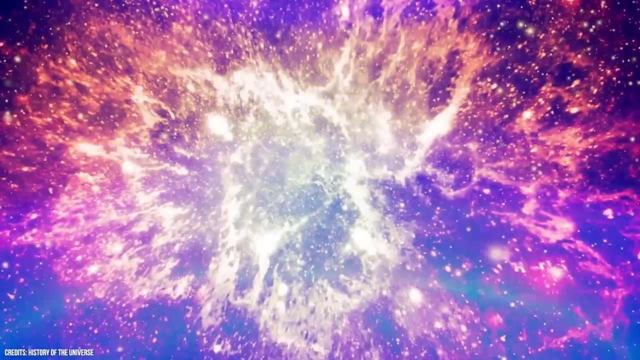 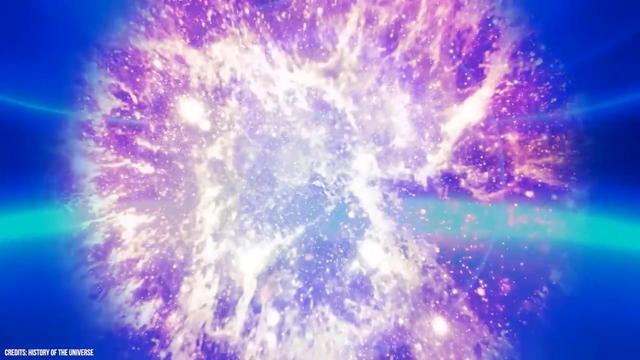 Is it reasonable to assume the existence of unobservable dimensions? However, the idea of additional dimensions poses intriguing questions and suggests observable phenomena. For example, we can imagine a massless particle that moves at the speed of light but traverses a compact dimension partially. 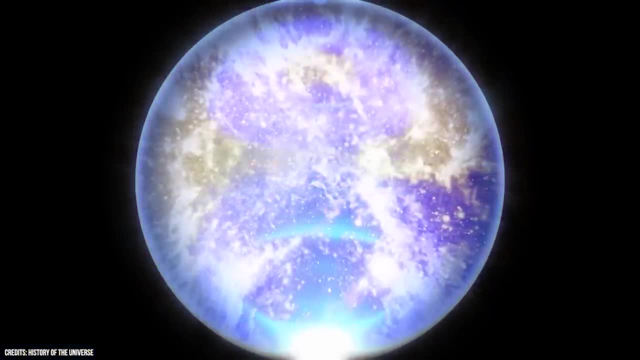 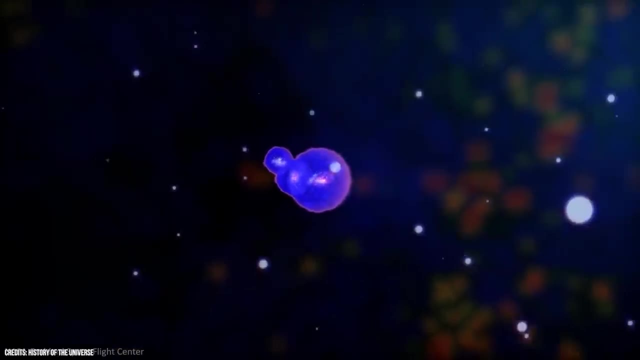 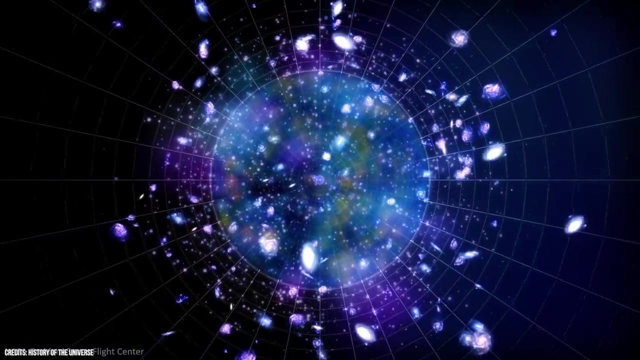 To us, this dimension remains unseen, resulting in a slower perceived motion akin to having mass. Additionally, compactified dimensions provide a simple mechanism for certain particles to exhibit significant mass. Currently, it requires excessive energy to create these particles in our particle accelerators. 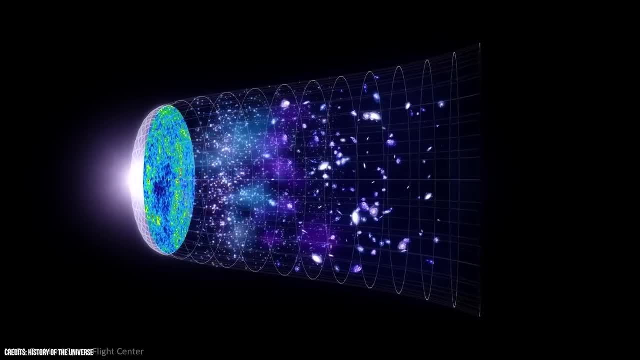 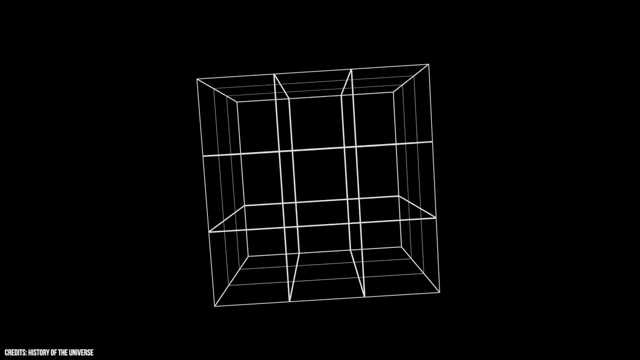 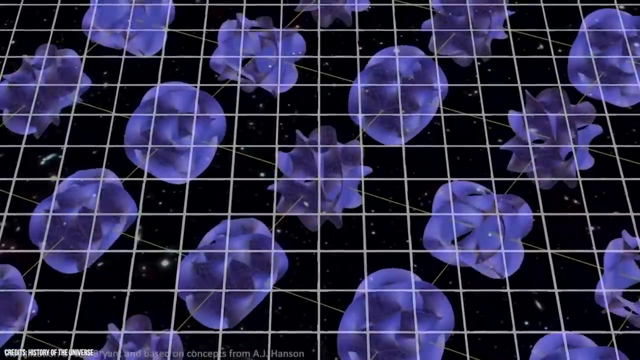 and confirm their existence. The presence of these extra dimensions also allows for a broader range of vibrational modes, leading to a greater diversity of potential particle types. Moreover, various ways of curling up the 6 dimensions predict different universes where strings adopt distinct vibrational modes. 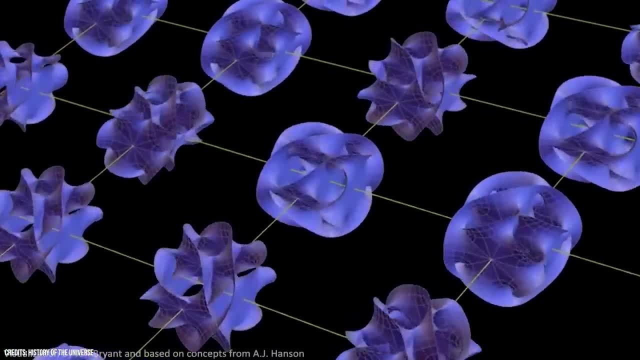 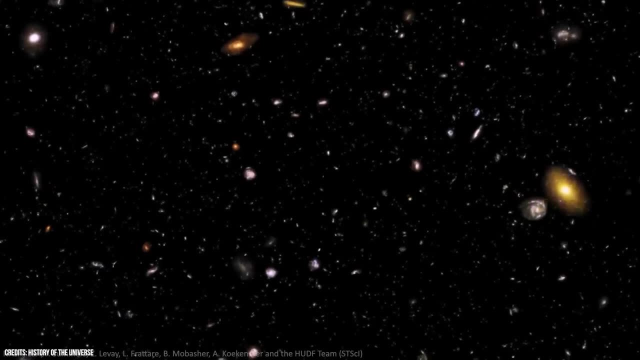 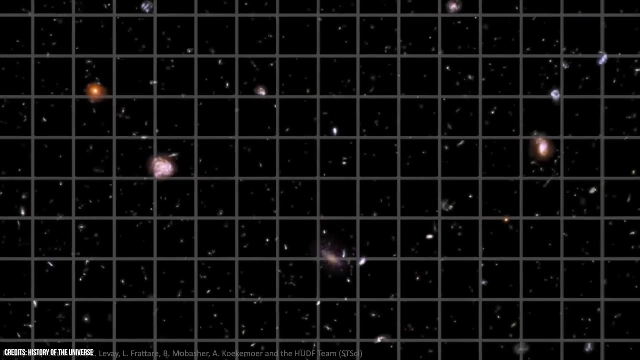 resembling different particles. By carefully selecting the compactification method, we can align our description with the observed particles in our world. However, amidst the multitude of possibilities, it remains unclear why our universe contains the particles of the Standard Model rather than an alternative arrangement. 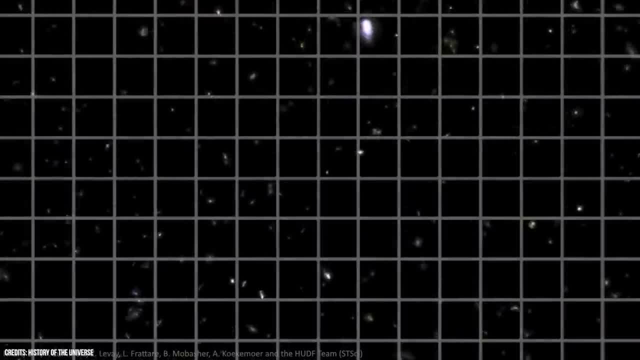 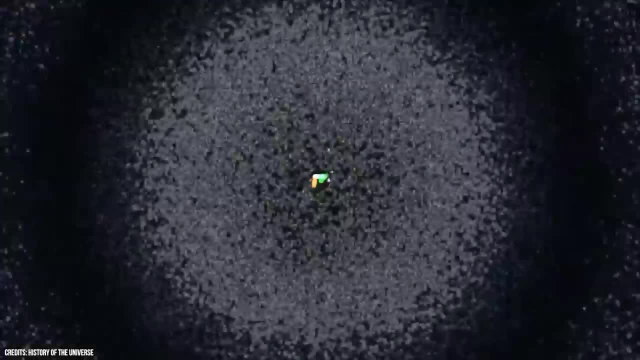 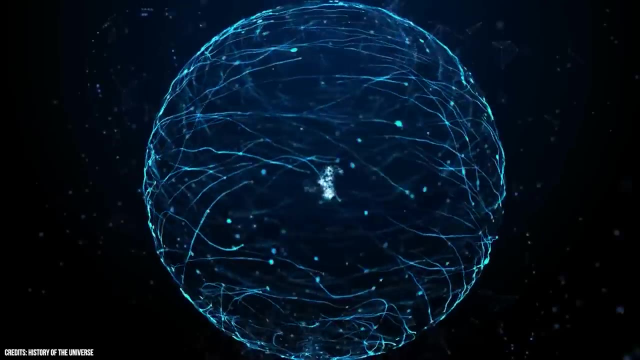 Speculative hypotheses suggest that the universe's geometry may have varied over time, transitioning between different compactifications. This transition could have altered the laws of physics during the universe's early stages. The string theory remains a speculative and challenging model to experimentally test due to the minuscule scale of strings. 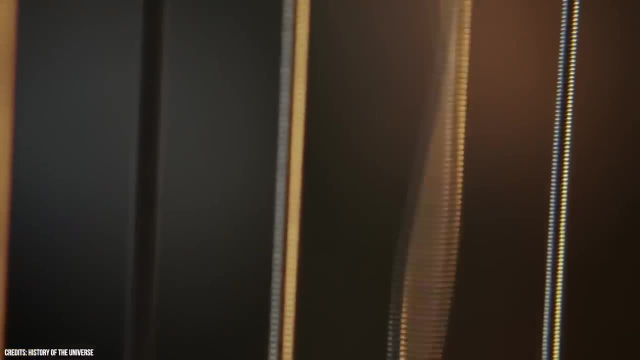 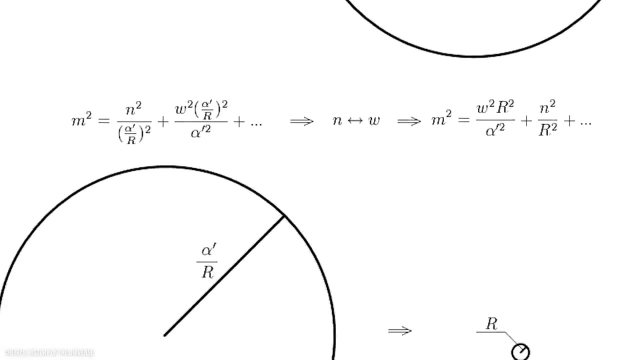 It's one approach among many in the pursuit of an ultimate theory. Nevertheless, it is one of the most promising models, surpassing its original goals. String theory enables us to describe quantum-scale gravity and explore black holes. It contributes to the development of mathematics. 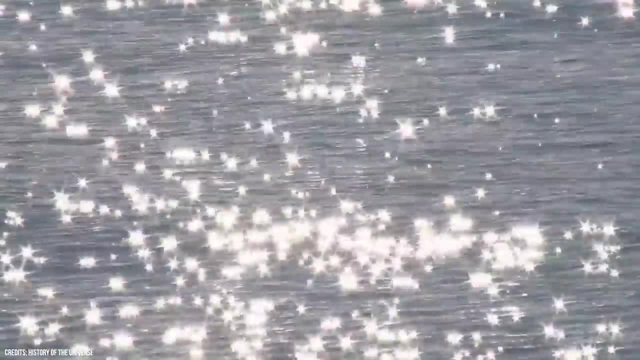 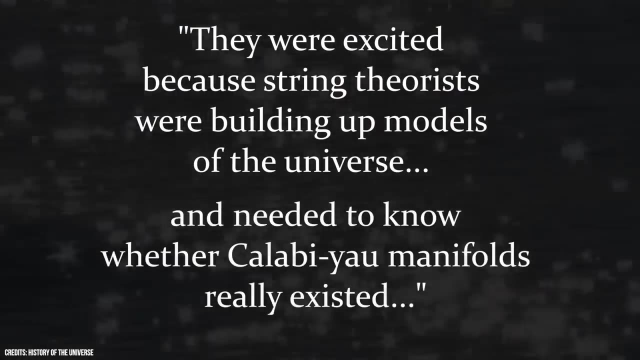 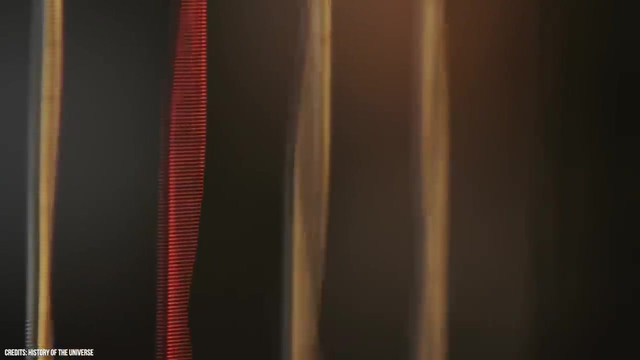 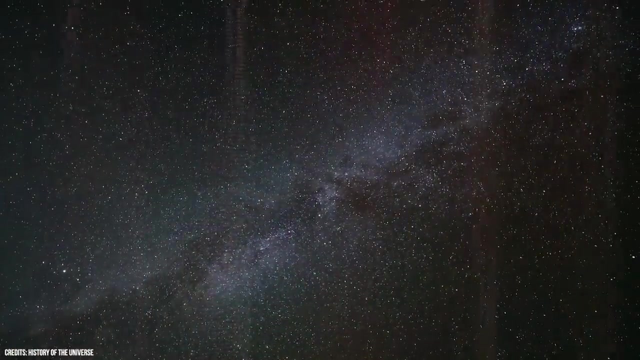 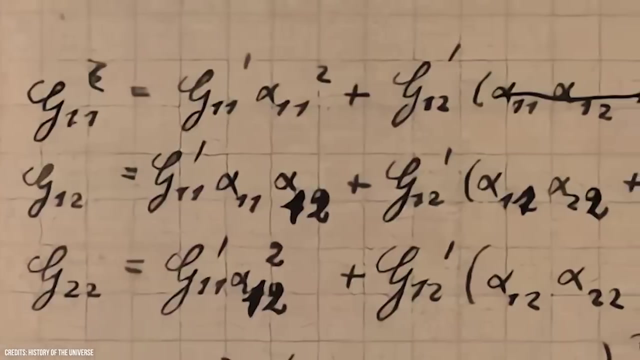 and enhances our understanding of the Standard Model. Additionally, it proposes hypothetical particles like axions as potential explanations for dark matter. Nonetheless, extensive research is still required. The aspects of string theory best understood heavily rely on supersymmetry, which suggests the existence of yet unobserved particles. 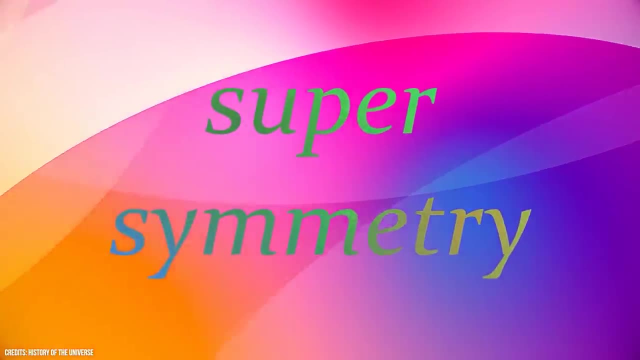 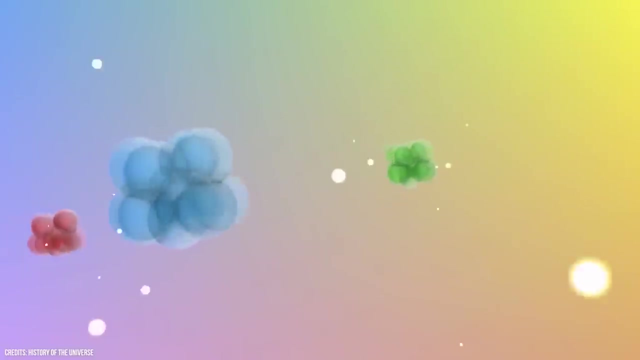 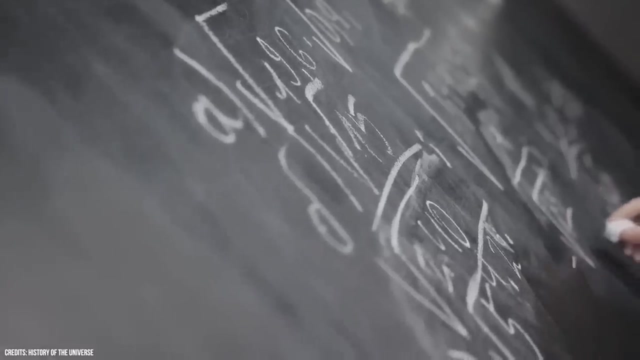 While some compactifications may explain the absence of supersymmetry, they remain rare and poorly comprehended. Lastly, it's worth noting that there are five distinct versions of superstring theory, each describing different types of universes. Mathematically, these theories approximate a more comprehensive model. 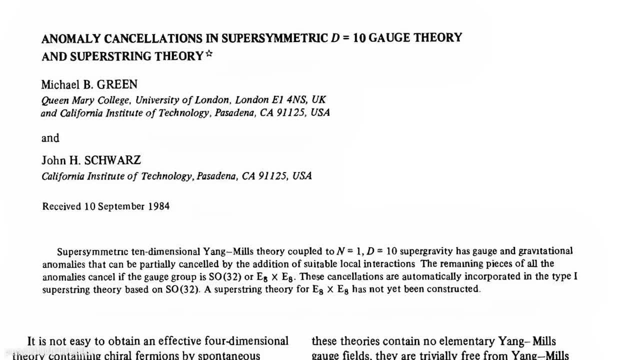 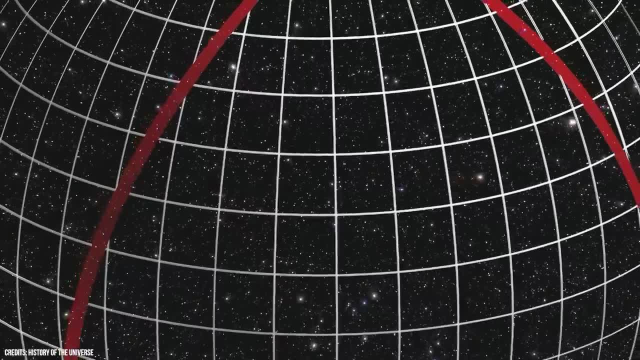 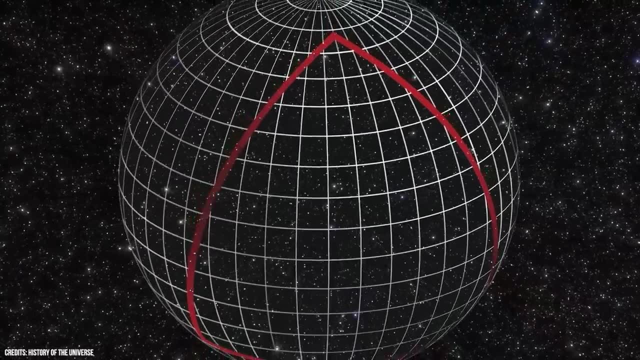 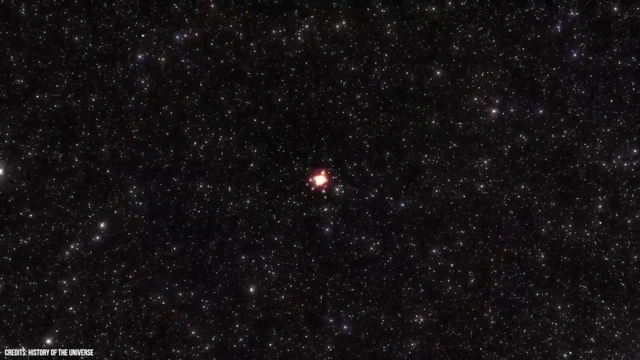 that describes an 11-dimensional universe. Now let's discuss why Roger Penrose says cosmic inflation is just a fantasy. The concept of cosmic inflation is a hypothesis proposed to explain certain observations of the early universe. Penrose's viewpoint stems from his alternative proposal. 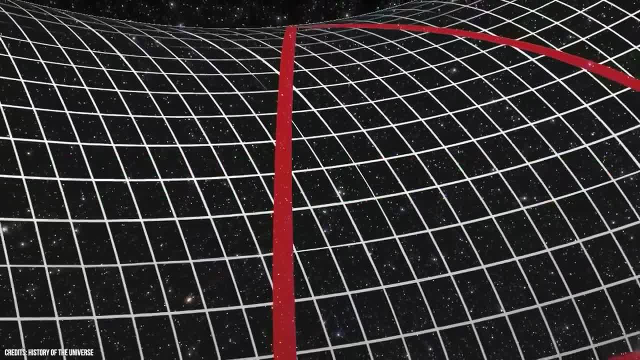 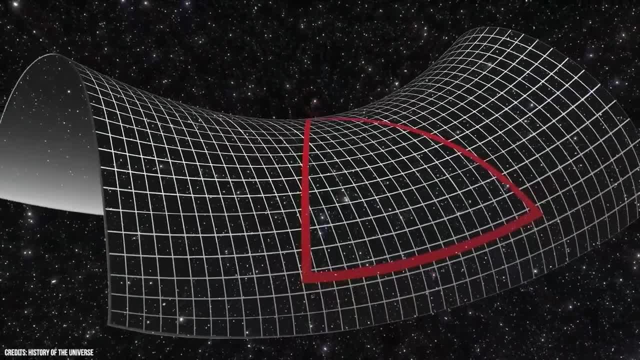 known as Conformal Cyclic Cosmology or CCC, which offers a distinct perspective on the origins and evolution of the universe. In Penrose's Conformal Cyclic Cosmology, the notion of an inflationary phase is challenged. 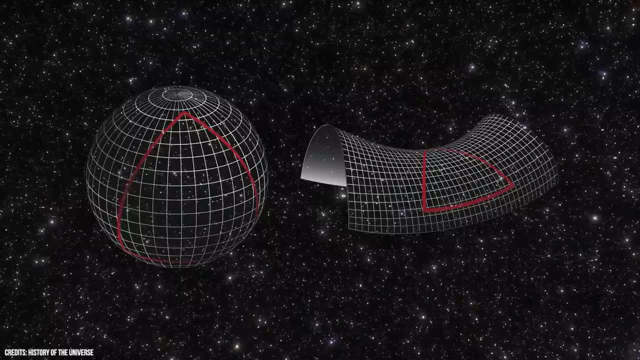 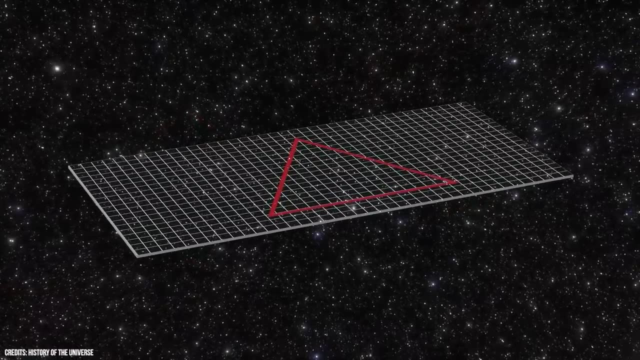 According to Cosmic Inflation, the universe underwent an extremely rapid expansion in the early stages, which resolved certain issues related to the observed uniformity. However, Penrose argues that the inflationary model introduces more questions than it answers. One of Penrose's main criticisms- 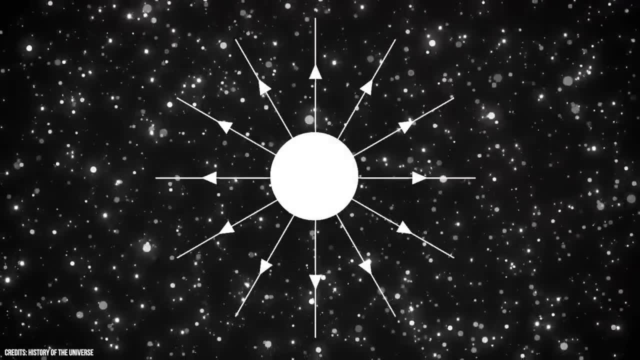 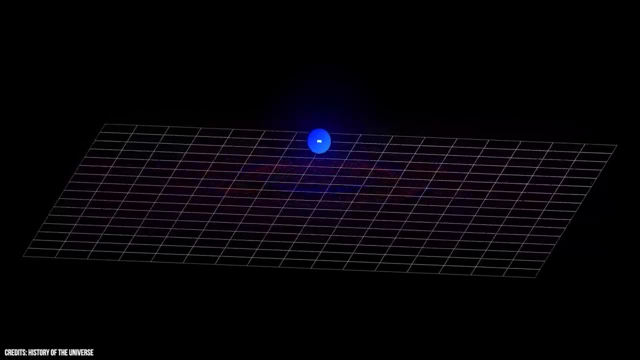 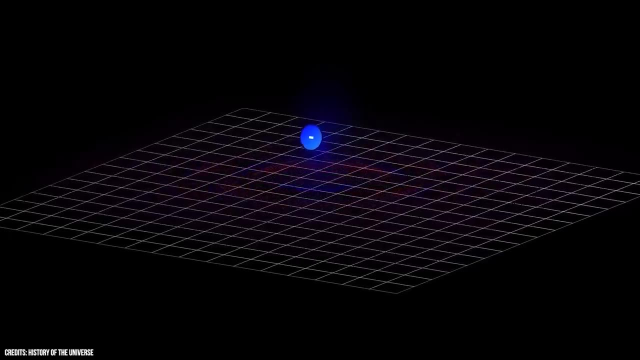 revolves around the lack of a satisfactory explanation for the initial conditions required for inflation to occur. Inflationary models typically rely on the assumption of a primordial scalar field that drives the expansion, but the origin and properties of this field remain largely speculative. Penrose questions the plausibility. 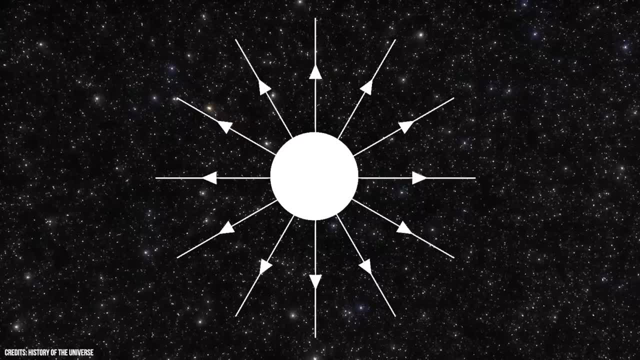 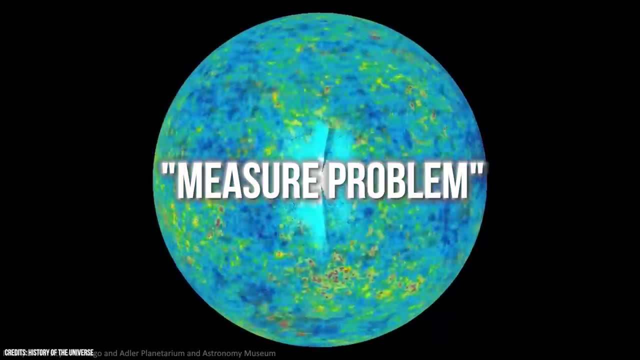 of such an expansion in the early stages of the universe. Penrose considers the plausibility of such assumptions and suggests they may be overly contrived. Another concern raised by Penrose is the so-called measure problem within the inflationary framework. Inflation predicts the existence of a multiverse. 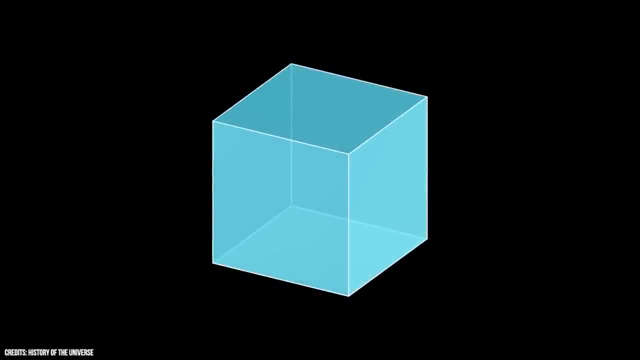 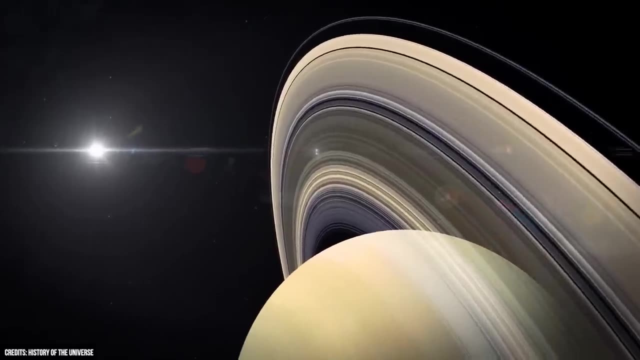 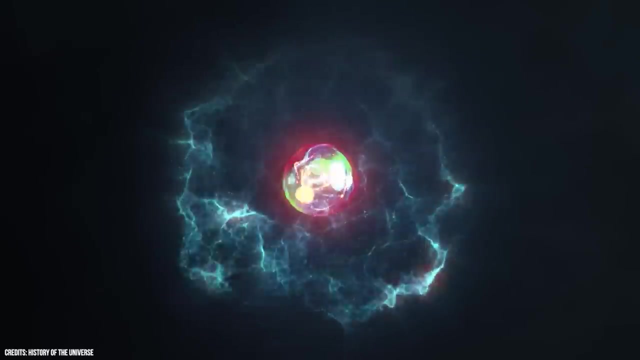 a vast ensemble of universes with different properties and physical laws. However, it becomes challenging to determine the probability distribution of universes within this multiverse and to explain why we observe the particular set of physical laws and constants that we do. Penrose argues that this lack of predictive power 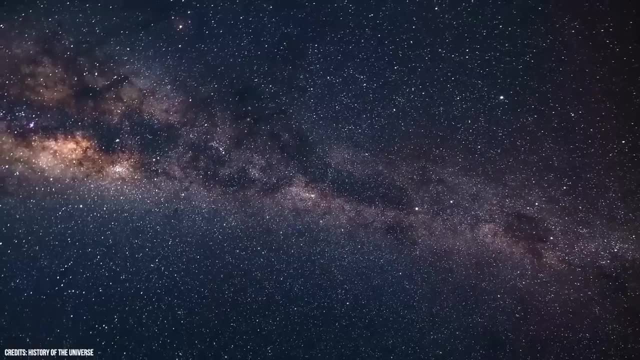 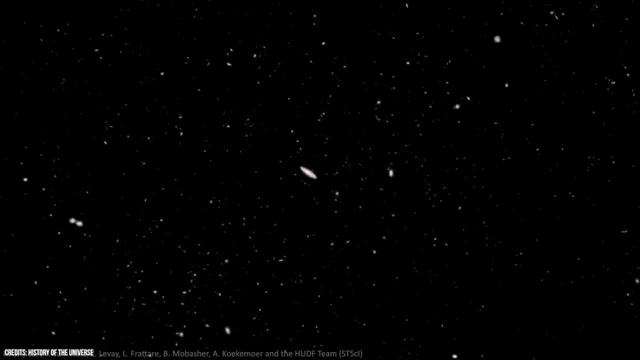 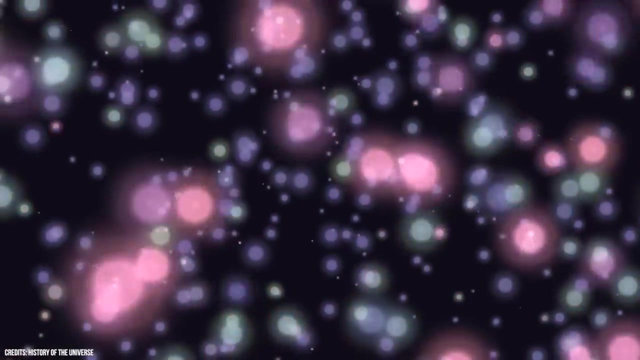 undermines the scientific rigor of inflationary cosmology. Additionally, Penrose's conformal cyclic cosmology proposes an alternative to the Big Bang singularity, suggesting that the universe experiences a cyclic series of expansions and contractions. According to this model, the universe undergoes a phase known as aeons. 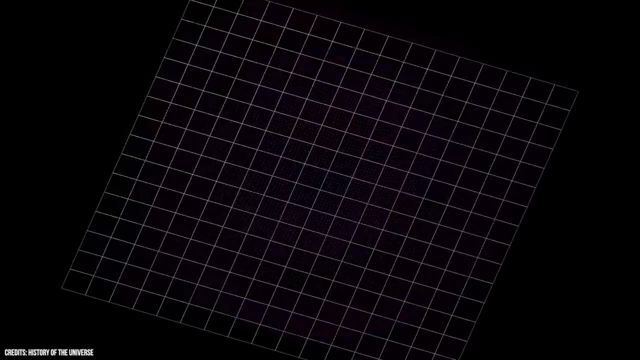 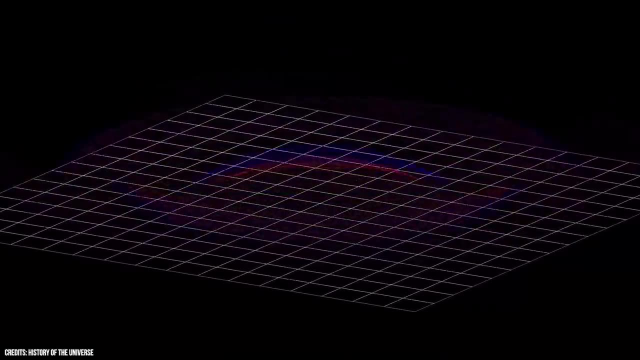 with each aeon preceded by a conformal phase that erases any remnants of the previous universe. In Penrose's view, this cyclic nature eliminates the need for an inflationary phase to explain the observed uniformity and flatness of the universe. I talk about things which are called aeons. 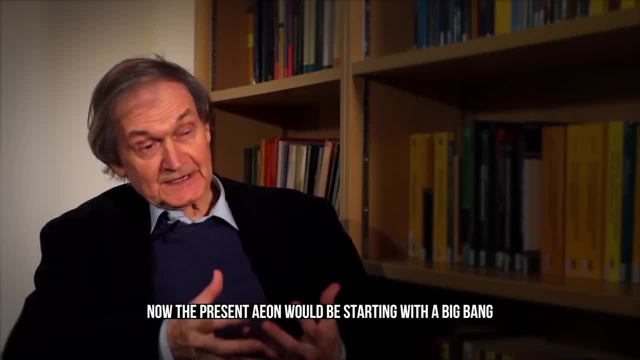 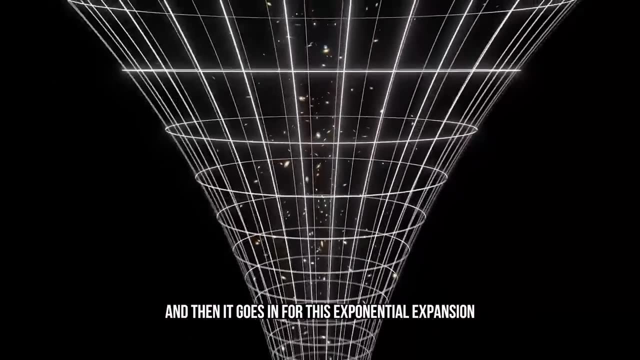 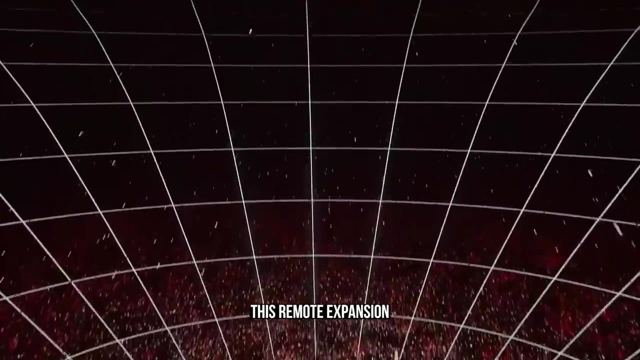 Now a present aeon would be starting with the Big Bang. the universe expands and then it goes into this exponential expansion which is fairly recently observed, and then that goes on forever. This remote expansion is physically equivalent to the expansion of the universe. 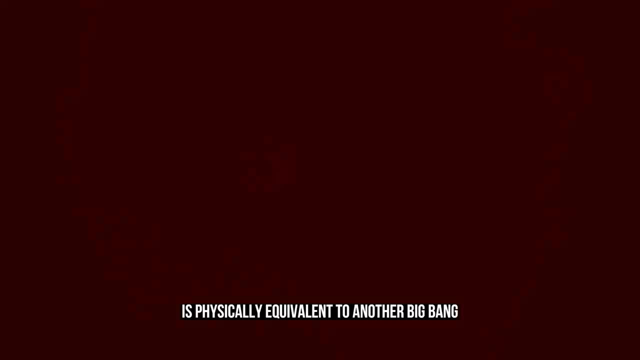 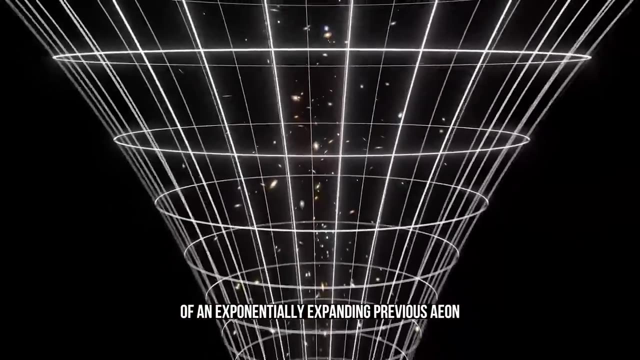 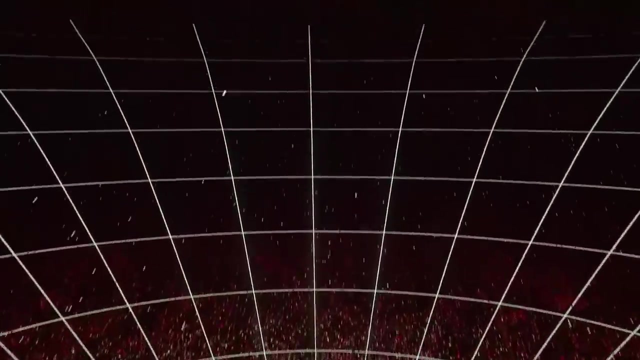 Physically equivalent to another Big Bang. And our Big Bang was the continuation of the remote future of an exponentially expanding previous aeon, And the idea is that aeons go on and on and on forever in both directions. Now let's explore Roger Penrose's research on black holes. 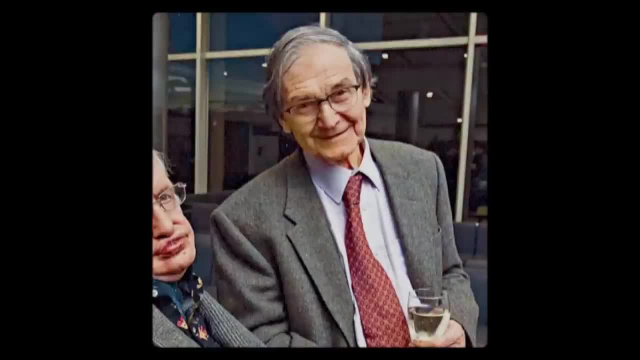 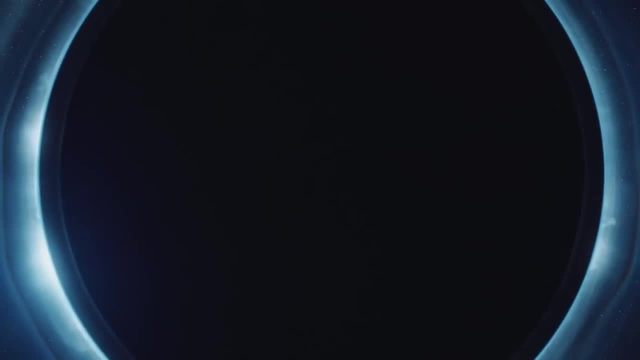 Penrose's exploration of black holes dates back to the 1960s, when he collaborated with Stephen Hawking to develop the singularity theorem. This theorem mathematically established the existence of singularities within black holes, regions of infinite density and curvature. 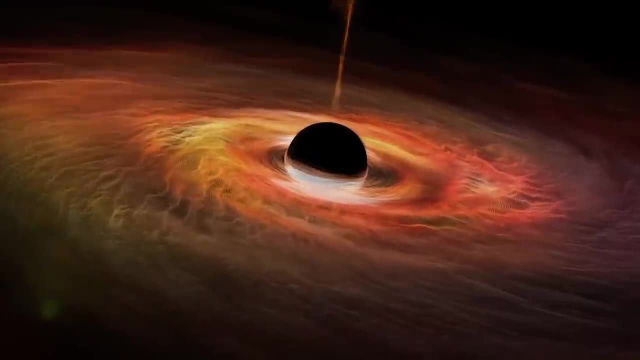 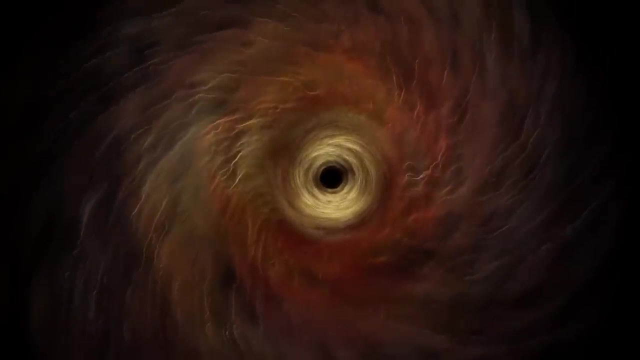 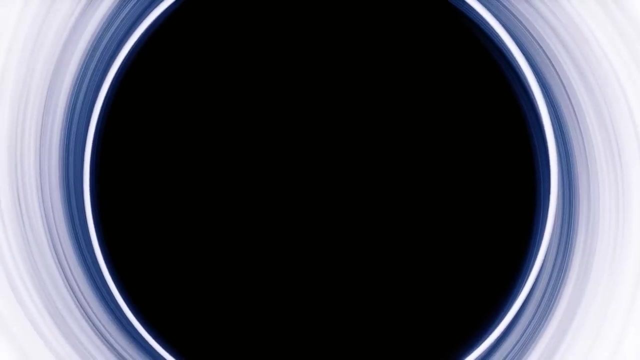 where the laws of physics break down. This groundbreaking work laid a solid foundation for the study of black holes and solidified their theoretical existence. One of Penrose's pivotal contributions to the black hole research is the development of the Penrose process. This process proposes the possibility. 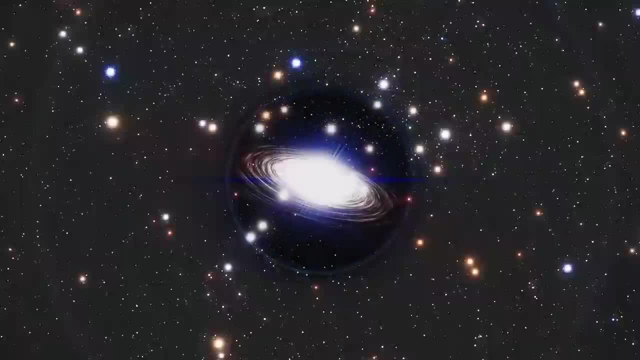 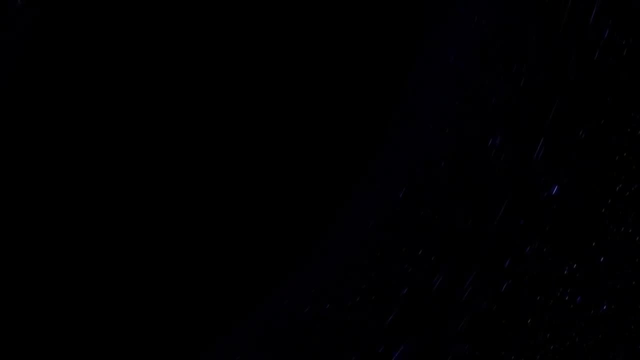 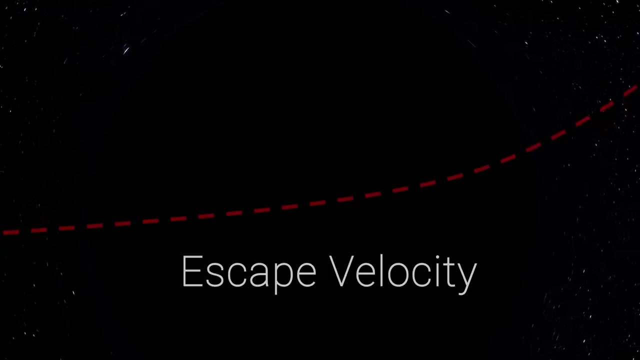 of extracting energy from a rotating black hole. According to Penrose, if an object or particle falls into the ergosphere, a region outside the event horizon but within the outer boundary of a rotating black hole, it can split into two components. One part falls into the black hole. 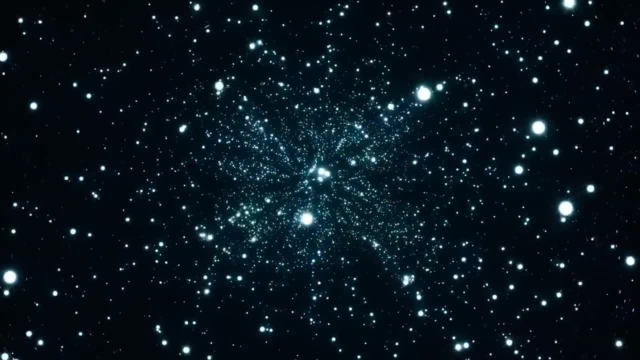 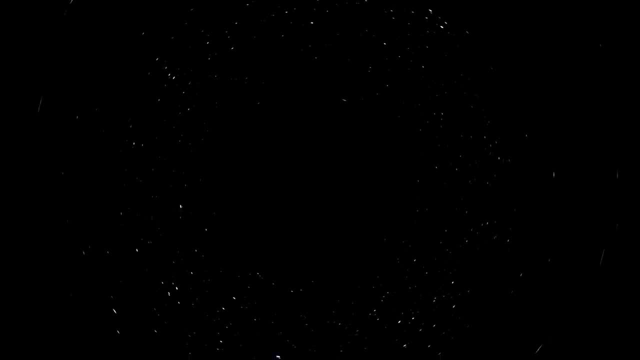 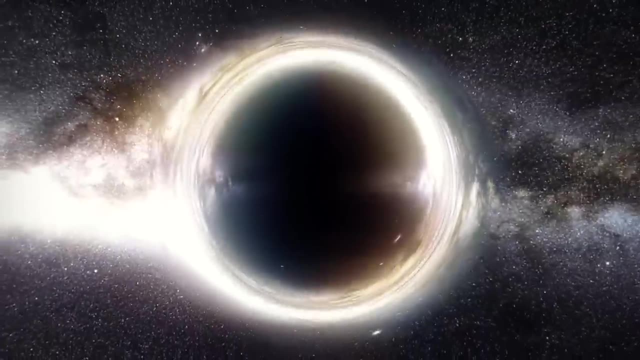 while the other escapes with increased energy. This concept implies that black holes could serve as immense power sources, harnessing the tremendous rotational energy stored within them. In addition to the Penrose process, Penrose introduced the concept of cosmic censorship. This hypothesis posits that 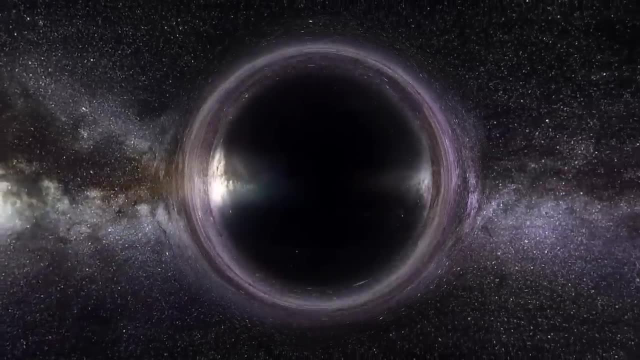 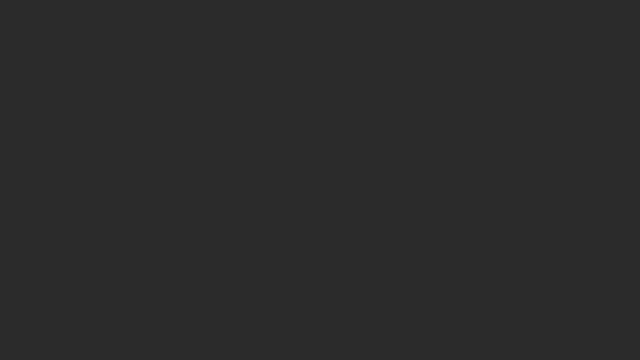 the singularities within black holes are always hidden from external observers by an event horizon, a boundary beyond which no information or signals can escape. This idea is rooted in the belief that the laws of physics should prevent naked singularities which would be visible to the outside universe. 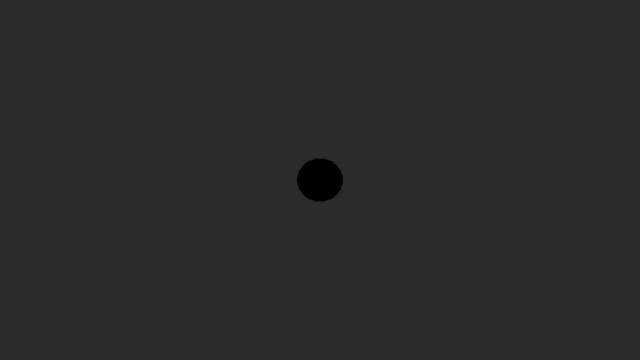 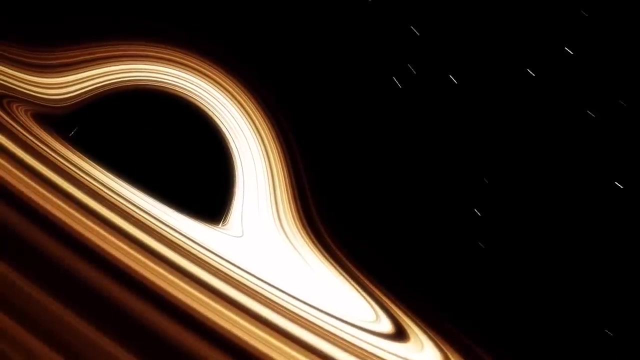 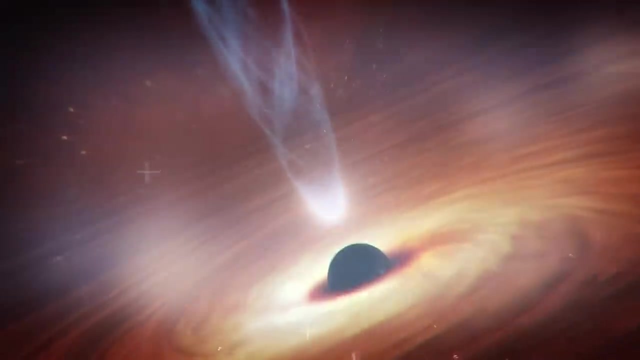 and potentially disrupt the fabric of space-time. While cosmic censorship remains an open question in astrophysics, Penrose's work has ignited extensive research and debate on this intriguing topic. Furthermore, Penrose's work on trapped surfaces has been a significant contribution to the study of black holes. 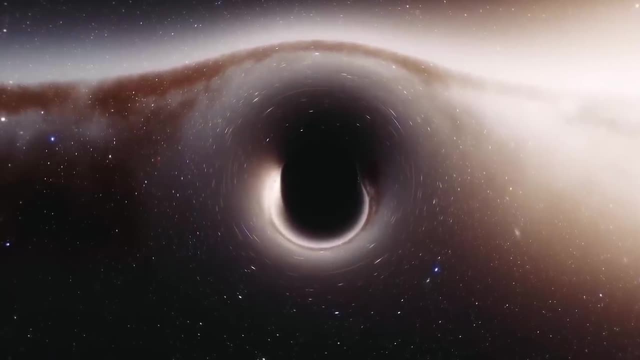 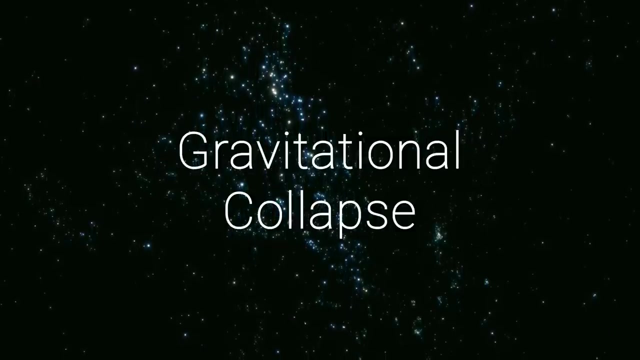 Trapped surfaces are surfaces in space-time that can capture light rays, preventing them from escaping. These surfaces play a crucial role in the process of gravitational collapse, where matter becomes increasingly compact until it forms a singularity within a black hole. Penrose's research on trapped surfaces. 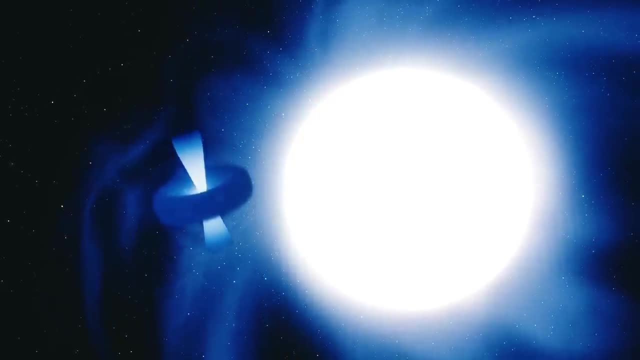 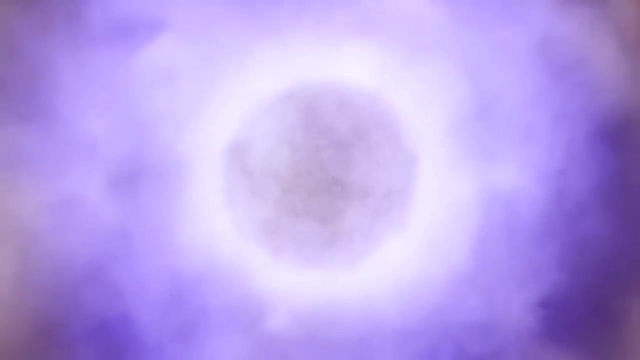 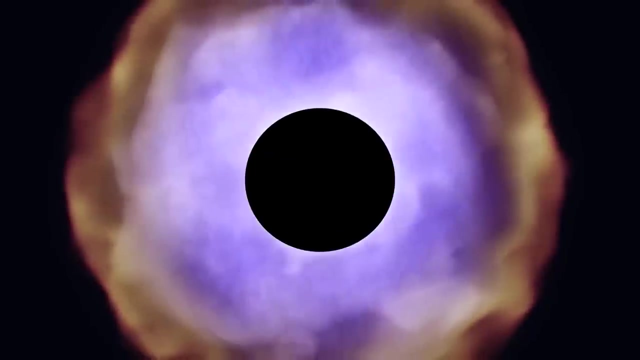 has provided valuable insights into the dynamics of black hole formation and has contributed to our understanding of the cosmic phenomena associated with them. Another notable aspect of Penrose's research on black holes is the proposal of the Cosmic No-Hair Conjecture. This conjecture suggests that the only properties 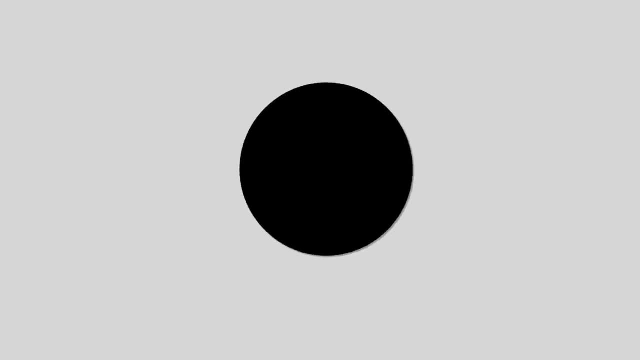 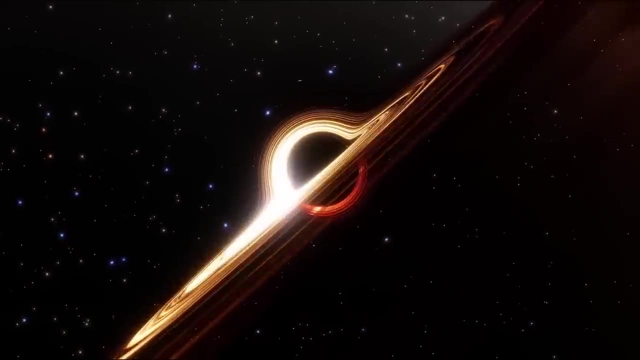 of a black hole that persist after its formation are its mass, electric charge and angular momentum. According to this notion, the specific details of the matter that formed the black hole, such as its shape or the nature of the material, do not have a lasting impact on its external properties. 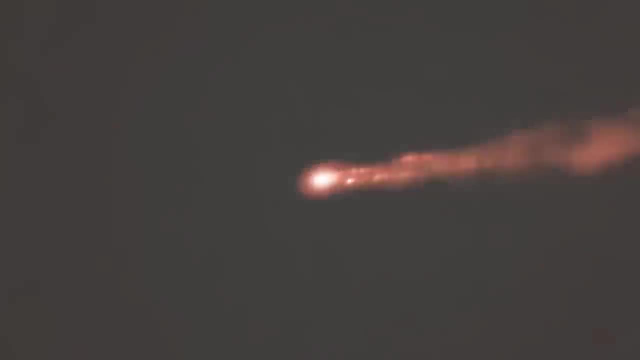 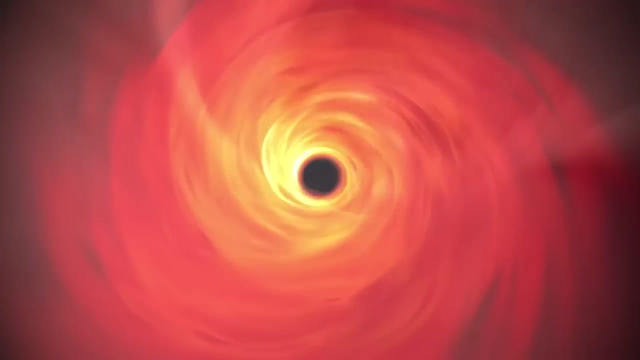 Instead, black holes are characterized solely by their global properties. The Cosmic No-Hair Conjecture has played a fundamental role in simplifying the study of black holes, allowing researchers to focus on their macroscopic features. Now let's explore some of the arguments put forth. 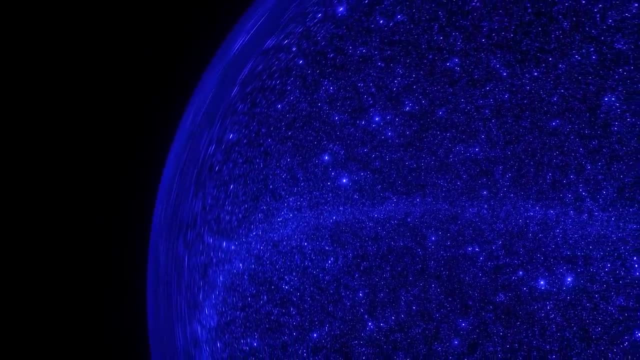 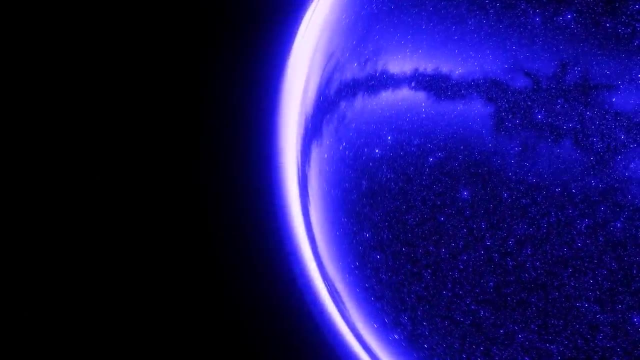 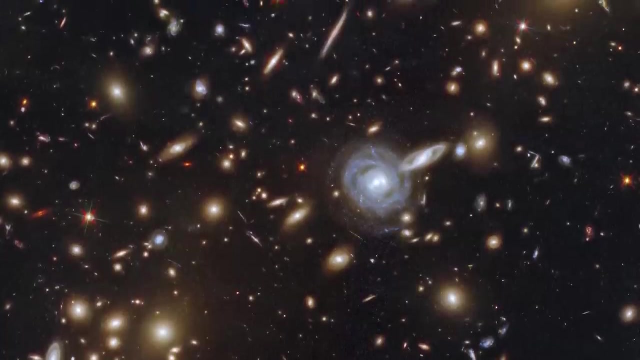 to suggest that dark matter might not exist. While the existence of dark matter is widely accepted within the scientific community as an explanation for certain astronomical phenomena, there are ongoing debates and alternative hypotheses that question its existence. One line of reasoning against dark matter posits: 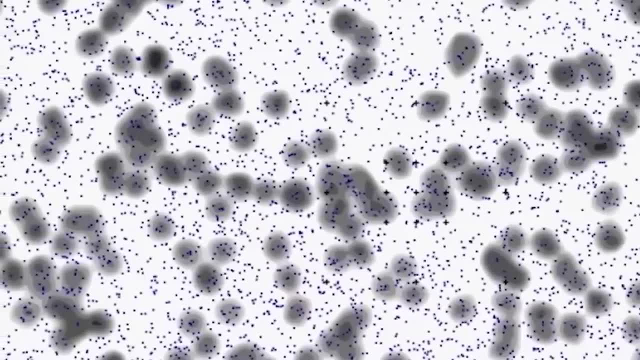 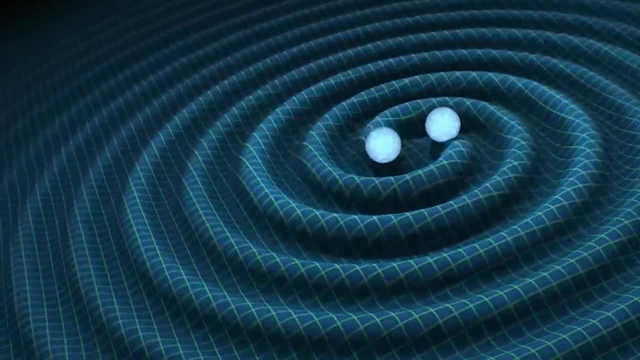 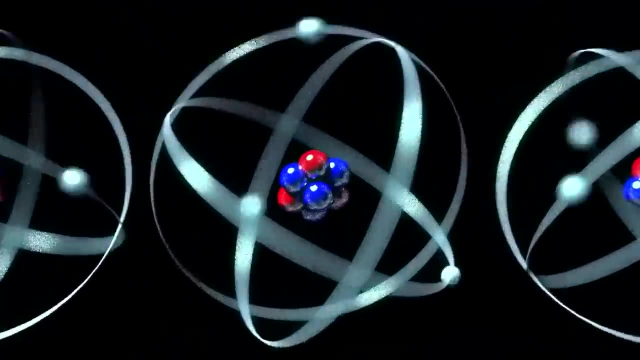 that the observed gravitational effects attributed to dark matter could potentially be explained by modifying our understanding of gravity itself. Instead of invoking the presence of invisible and non-interacting matter, proponents of modified gravity theories argue that our current understanding of gravitational forces may be incomplete. 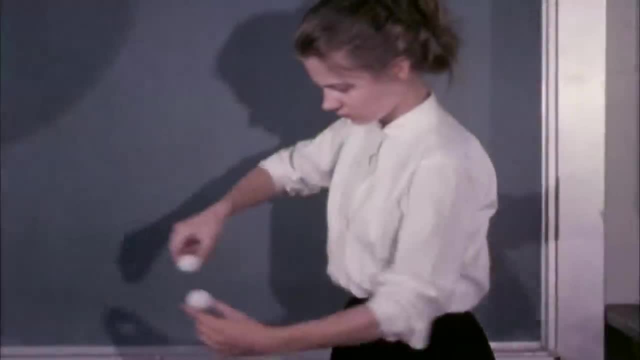 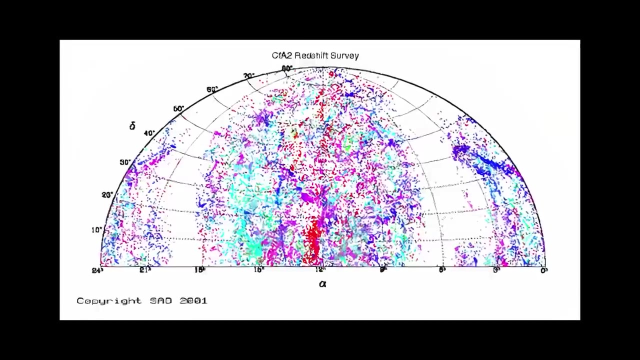 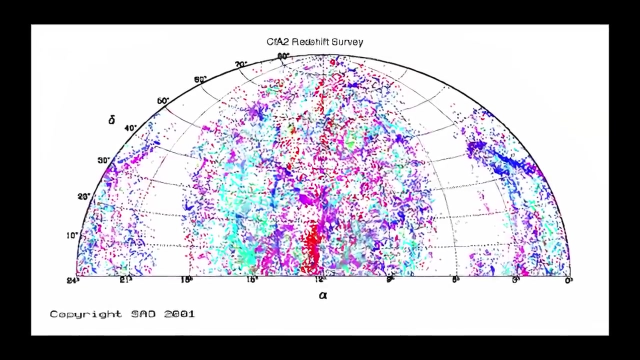 These alternative theories propose modifications to the laws of gravity at large scales, such as modifications to general relativity, to explain the observed phenomena without the need for dark matter. Another argument against dark matter stems from the lack of direct observational evidence, Despite extensive efforts. 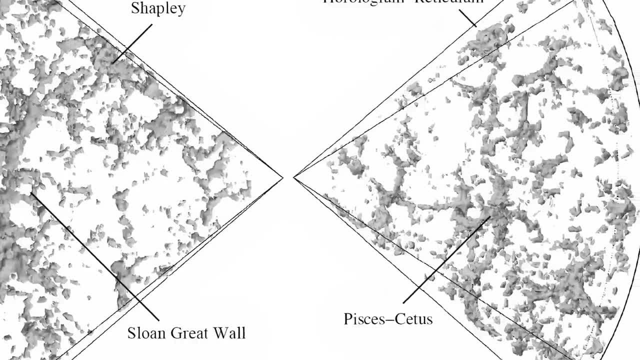 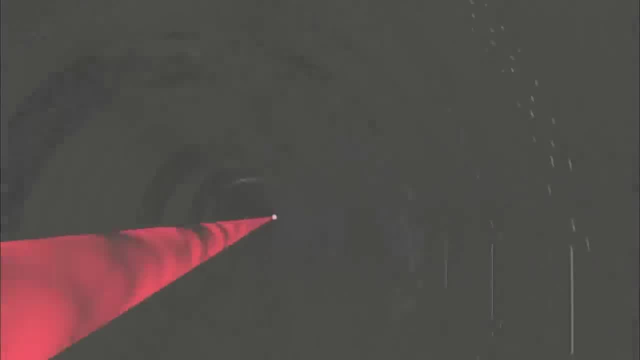 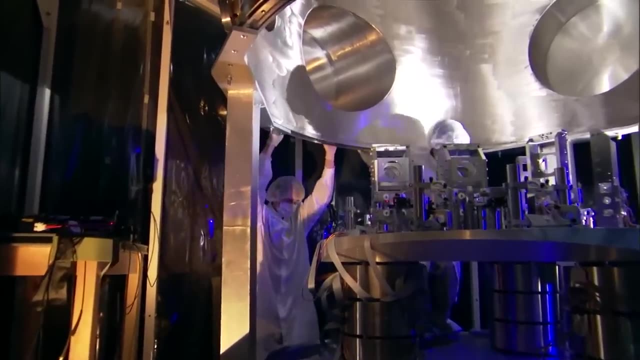 no direct detection of dark matter particles has been made to date. Various experiments, such as those involving particle detectors and underground laboratories, have been conducted in the search for dark matter particles. However, these experiments have not yielded definitive evidence for the existence of dark matter. 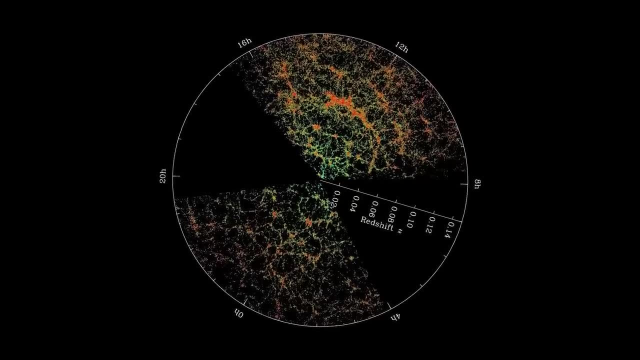 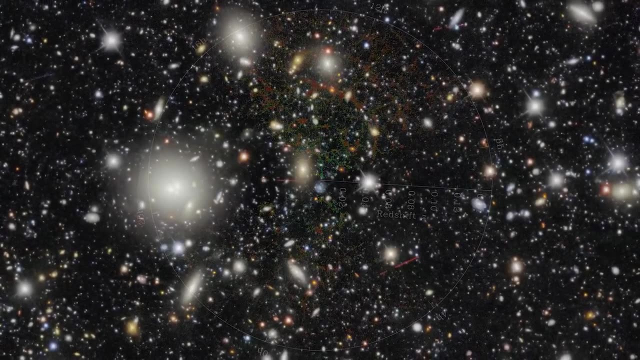 Critics argue that this absence of direct detection casts doubt on the existence of dark matter as a distinct form of matter. Additionally, some researchers argue that the observed gravitational effects attributed to dark matter could be the result of other astrophysical phenomena rather than the presence. of an entirely new form of matter. For instance, gravitational interactions between visible matter, such as stars and gas clouds within galaxies, could potentially account for the observed effects without invoking dark matter. This viewpoint suggests that our understanding of the dynamics of visible matter might be incomplete. 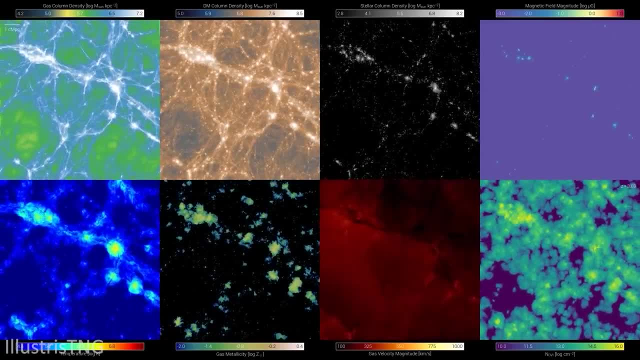 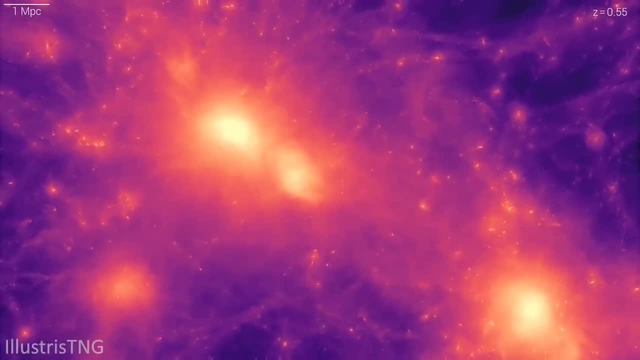 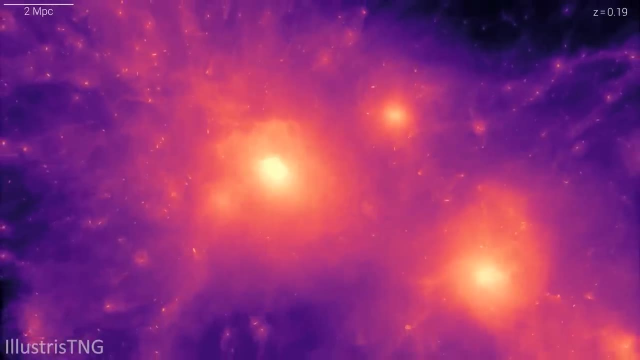 or that other astrophysical mechanisms are at play. Furthermore, critics of dark matter question its role in explaining certain observations such as the rotation curves of galaxies. They propose alternative explanations, such as modifications to the distribution of visible matter or the presence of unseen baryonic matter. 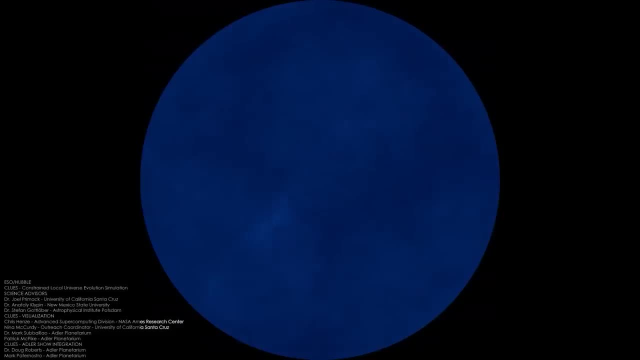 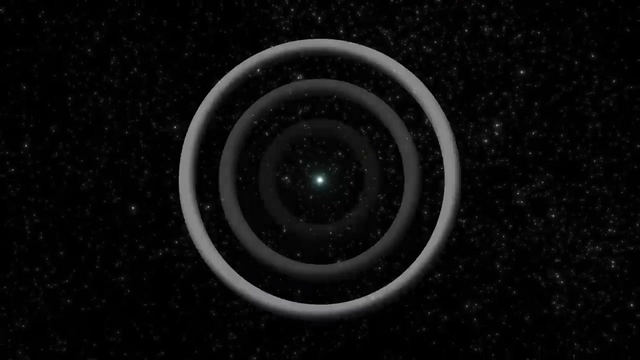 to account for these observations without invoking dark matter. These alternative hypotheses seek to address the discrepancies between the predicted and observed behavior of galactic rotational curves, suggesting that dark matter might not be the only viable explanation. It is worth noting that the arguments against dark matter 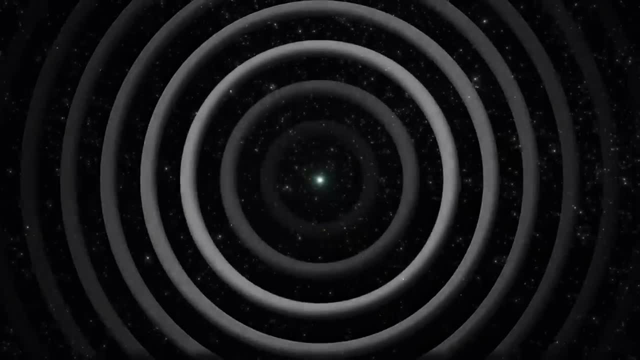 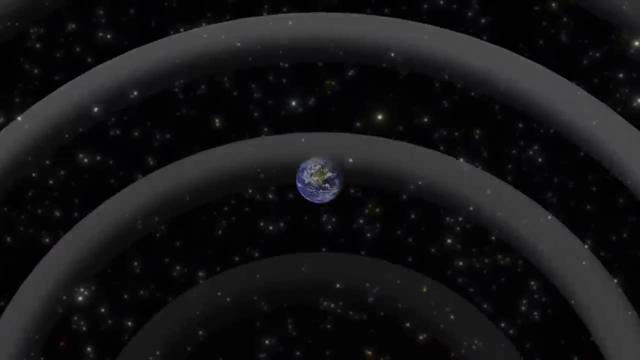 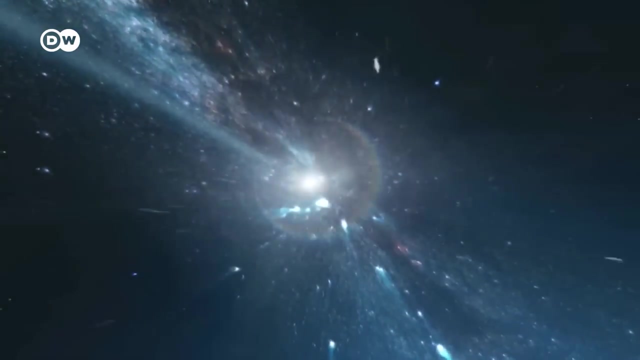 are not yet widely accepted within the scientific community And they remain subject to ongoing debate and scrutiny. Many physicists and astrophysicists consider the dark matter to be the most compelling explanation for a range of phenomena, including galaxy rotation curves, gravitational lensing. 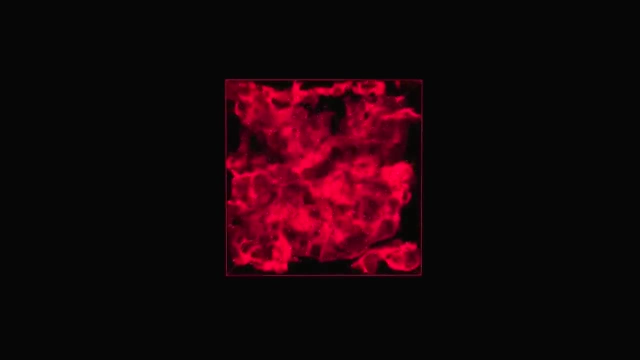 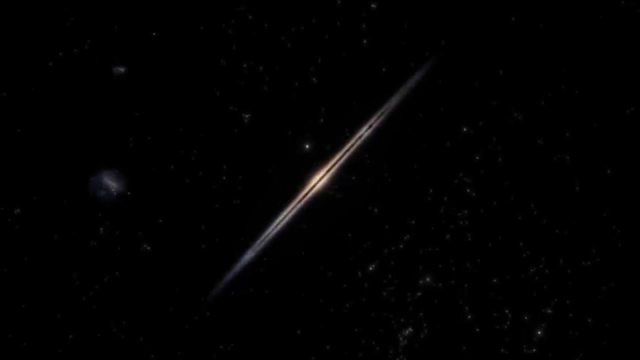 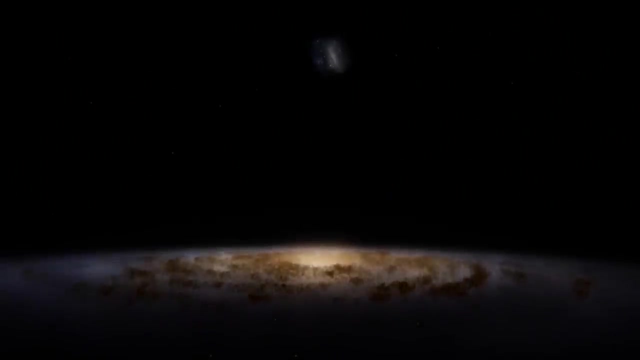 and the large-scale structure of the universe. Numerous observations and simulations strongly support the existence of dark matter as a significant component of our universe. While the critiques against dark matter offer alternative perspectives, they have not yet provided a comprehensive and widely accepted explanation for the observed phenomena. 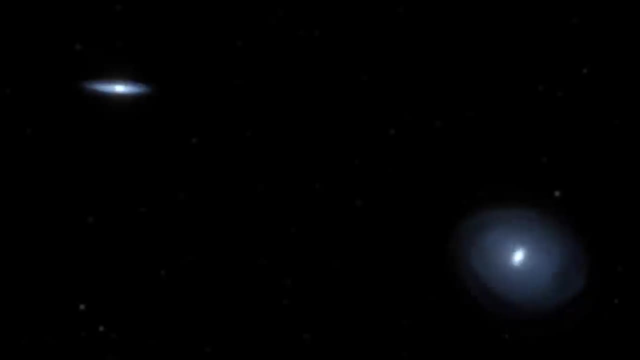 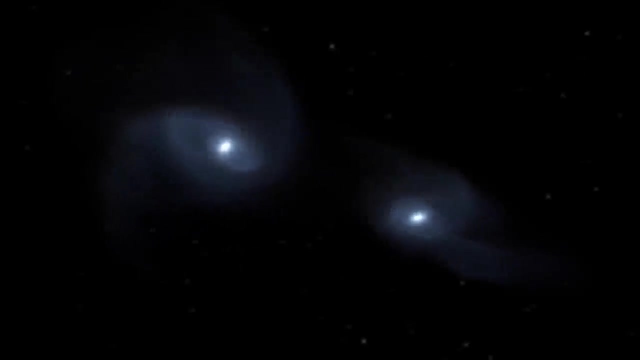 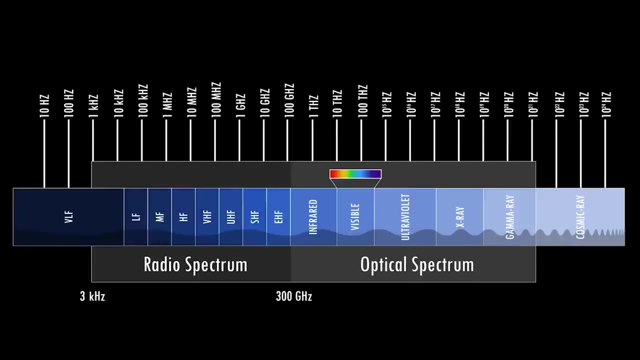 that dark matter successfully accounts for Dark matter remains the prevailing hypothesis that best fits the available evidence and provides a consistent explanation for a range of astrophysical observations. If dark matter does not exist, it will pose a profound challenge to our current understanding of the universe. 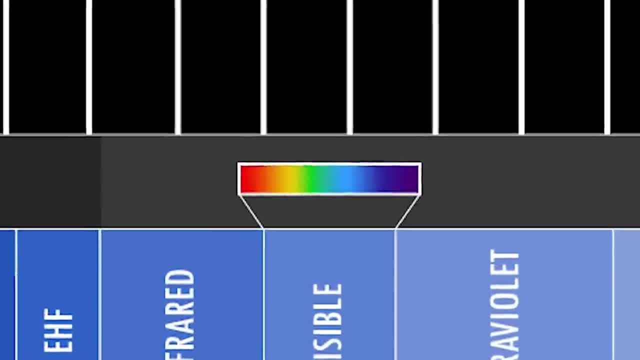 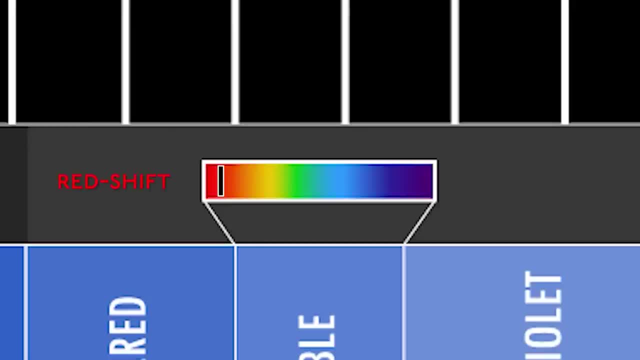 Despite its elusive nature, its existence has been inferred through its gravitational effects in the dark matter and the cosmic microwave background. Without dark matter, one of the key pillars of the standard model of cosmology would crumble. Dark matter's presence is thought to explain. 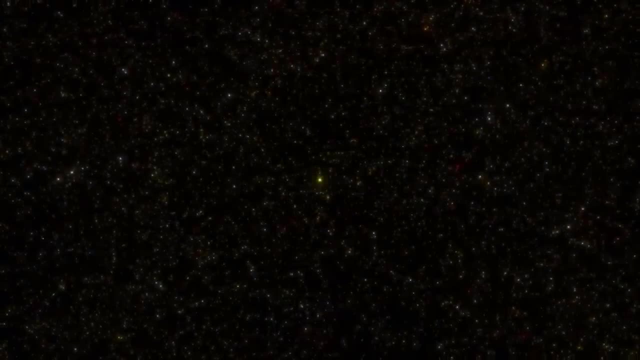 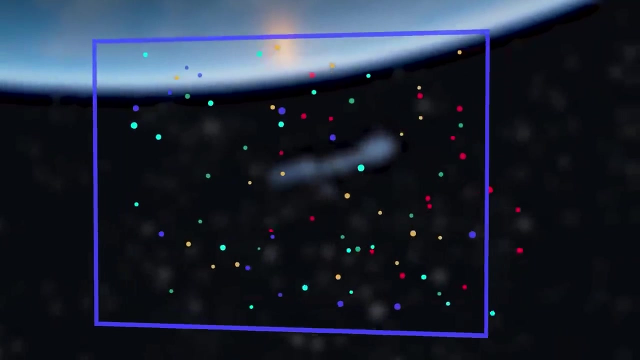 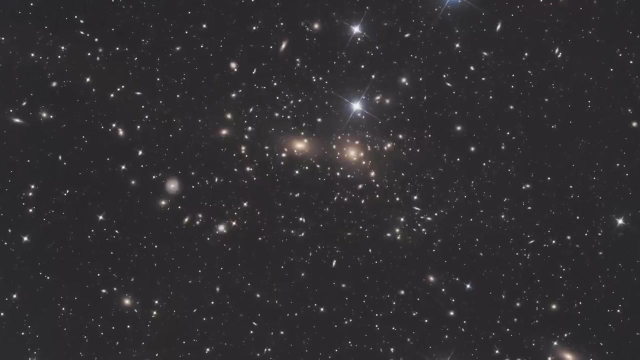 the observed rotation curves of galaxies, the large-scale structure of the universe and the gravitational lensing effects. If it were absent, these phenomena would demand an alternative explanation. Scientists might need to revise their theories of gravity, seeking new fundamental laws to account for the observed effects. 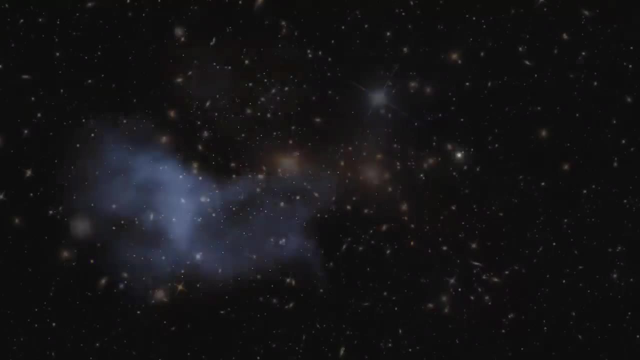 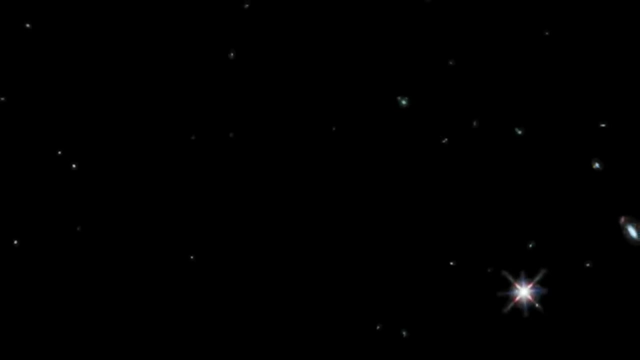 Modified Newtonian dynamics is one such approach, but it has not fully explained all the observations as successfully as the dark matter model. The absence of dark matter could also imply that our understanding of the universe's early evolution might be flawed. as dark matter plays a crucial role, 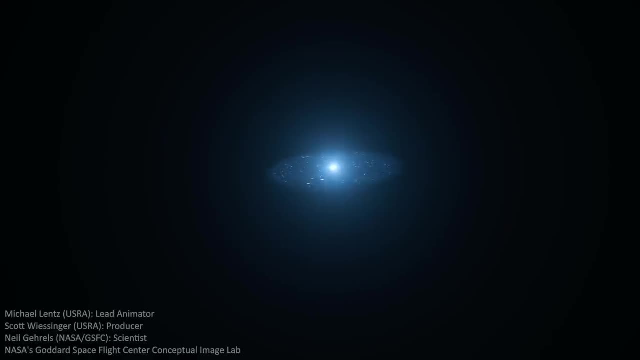 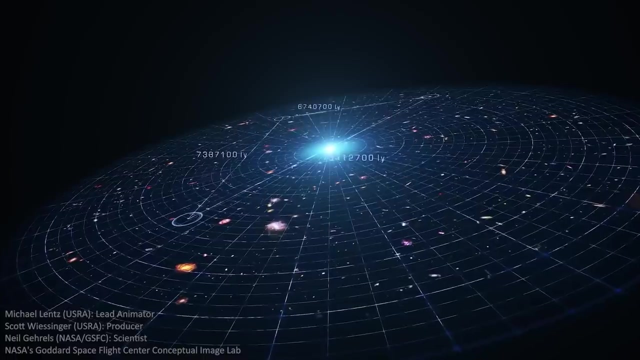 in shaping the distribution of matter during cosmic structure formation. So that seems enough for this video. We hope you enjoyed watching it. If so, give this video a thumbs up and leave a comment to let us know your thoughts. We'll be back with another amazing video. Until then, thanks for watching.